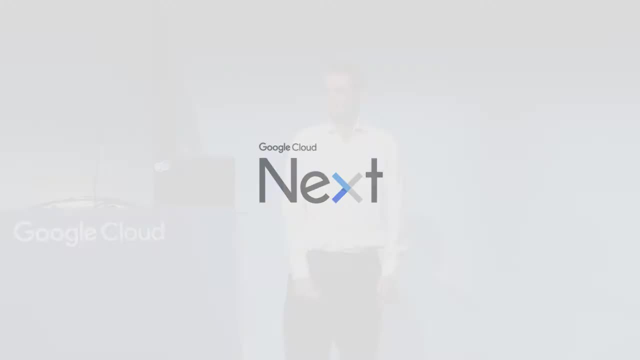 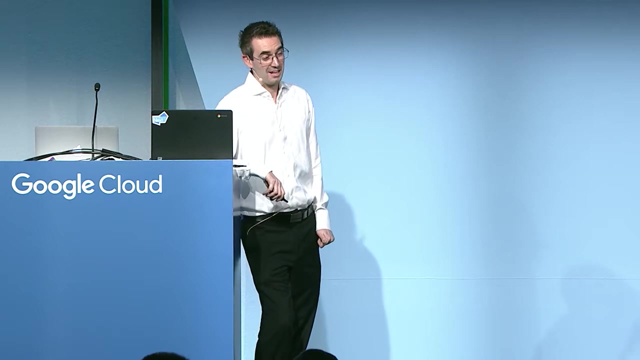 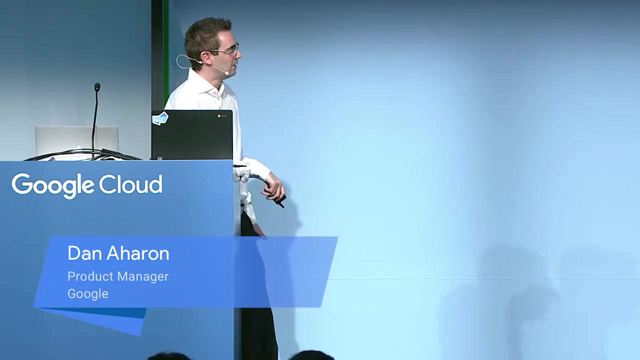 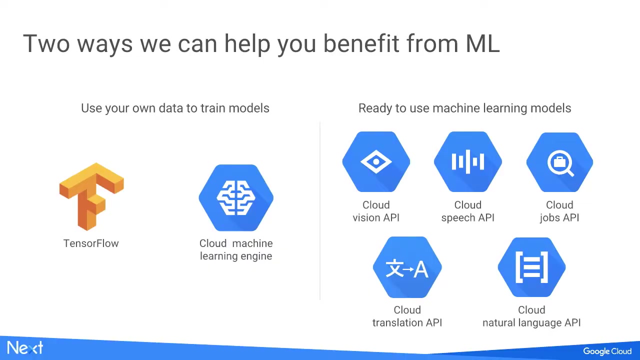 I'm excited to be here at Google Cloud Next talking to you about a topic that I'm very excited about: speech recognition. Hope you're having a great time here at Google Cloud Next. So why do we even have speech recognition at Google Cloud Platform? So we started developing. 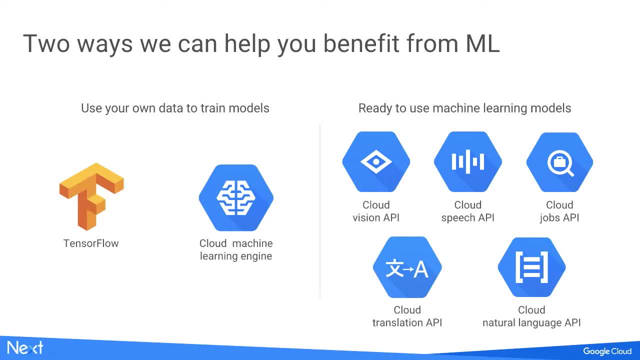 speech recognition at Google more than a decade ago- I think even more than 15 years ago- And we did it for our internal uses, for web search and later for our other apps, because we figured that voice will be used very frequently. It's very prominently in our apps, but we never intended to offer it to third parties. 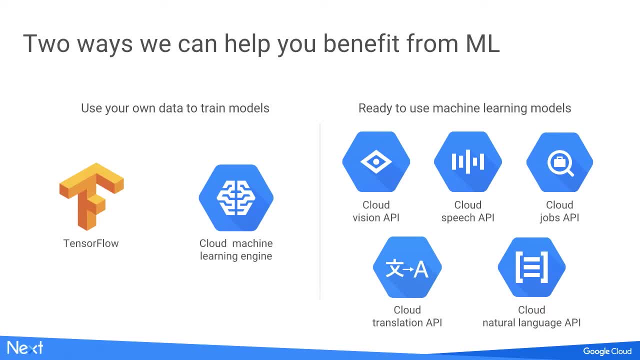 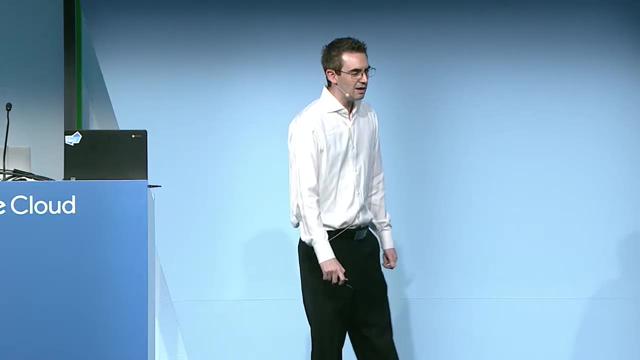 as a commercial service And that changed last year And the reason why that changed was we went through a big revolution at Google with machine learning. I'm sure you've heard a lot about it in our keynotes this year and last year And we really wanted to help other. 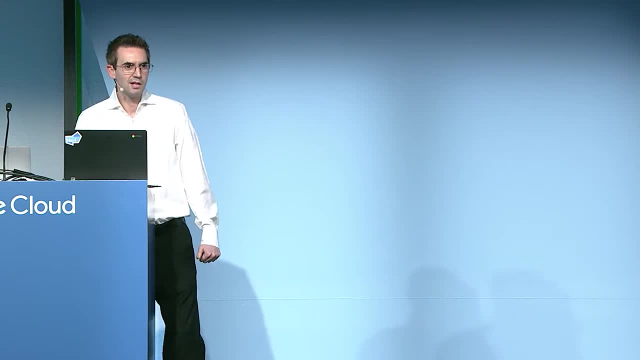 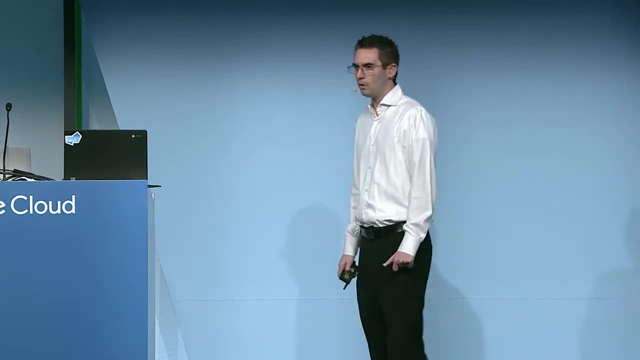 companies take advantage of machine learning and benefit the same way that we did, And we're doing that in two different ways. One way is we're helping companies build their own custom machine learning models, And anyone can use TensorFlow- It's open source, Just. 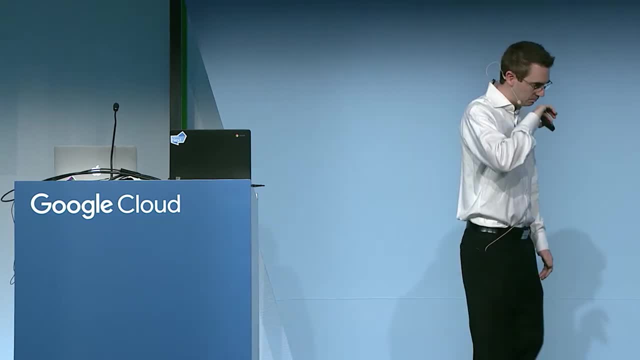 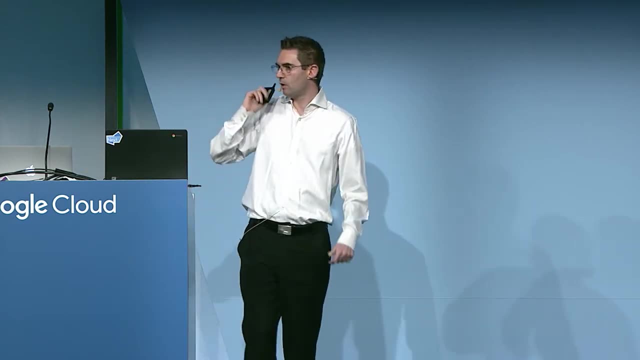 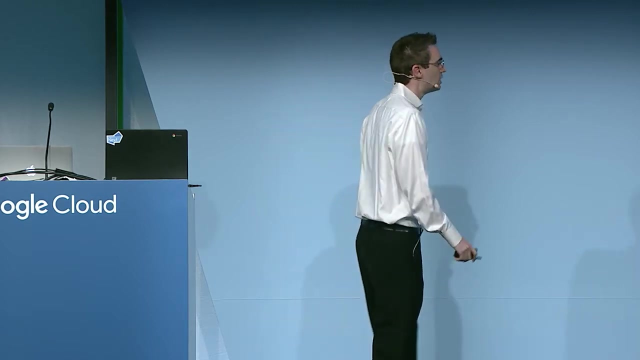 download it for free and start using it right away. Sorry, Or we started offering in beta in September, And yesterday we announced general availability for Cloud Machine Learning Engine, which lets anyone use machine learning on their own And it's very easy to use, And. 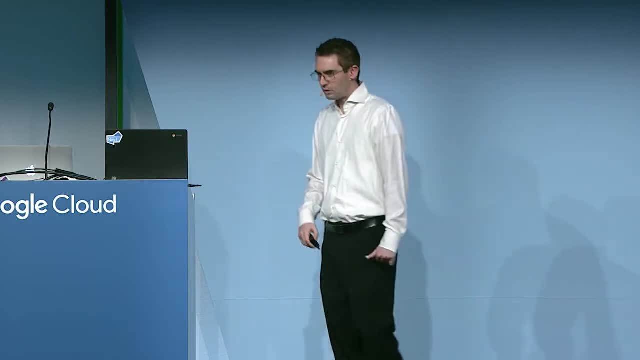 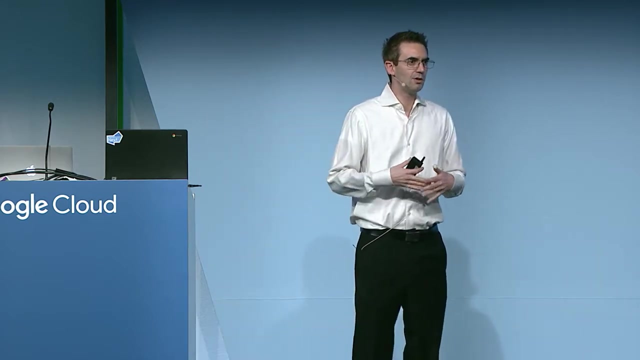 it's very easy to use on the cloud to develop their own models. So that's very exciting And we think over time that's going to enable a lot of new opportunities, different use cases for businesses. But the reality is that most businesses don't have sort of the expertise. 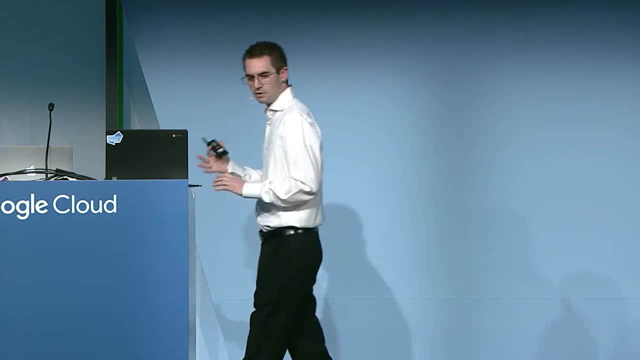 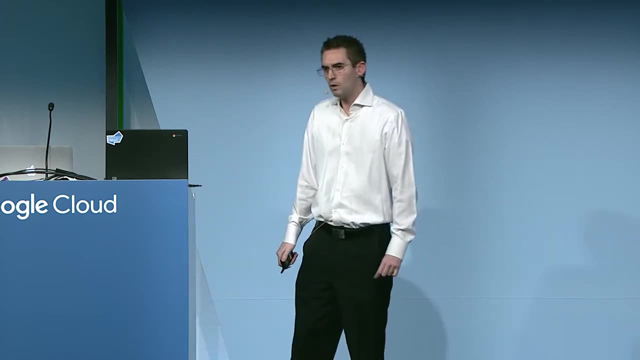 or the resources or the data that is needed to develop their own custom models. And in our aspiration to still enable people to take advantage of machine learning, we also offer what we call our machine learning machine learning model, And that's what we call machine 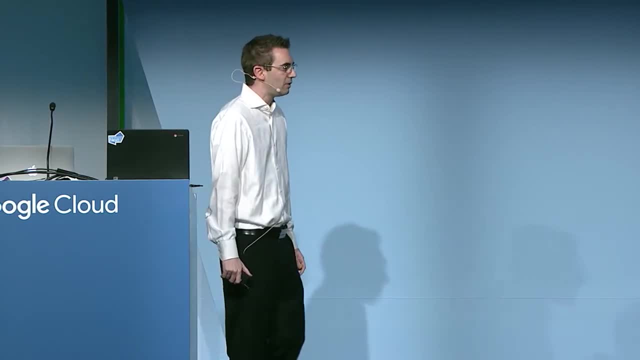 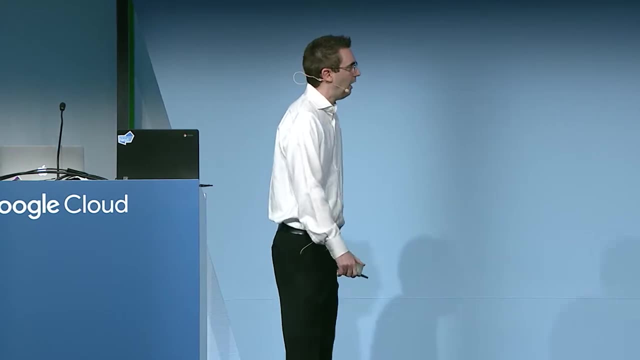 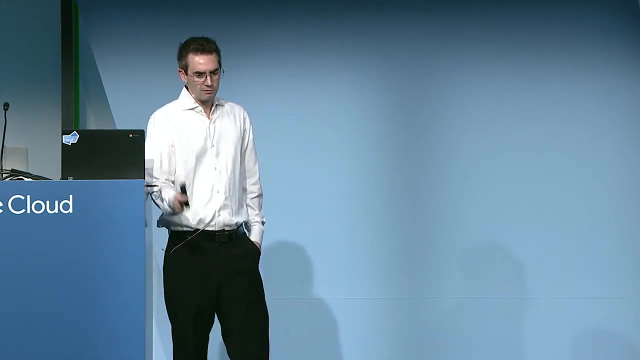 learning APIs, So ready to use, models that anyone can just use as an API, as a service that we've already pre-trained. And in that set we have cloud vision, cloud speech, cloud jobs, cloud translation, natural language API. And then yesterday we added one more: 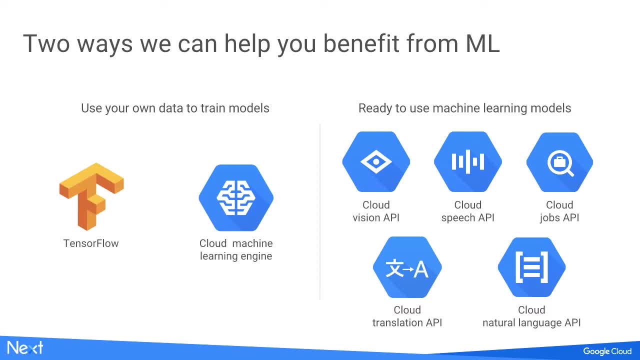 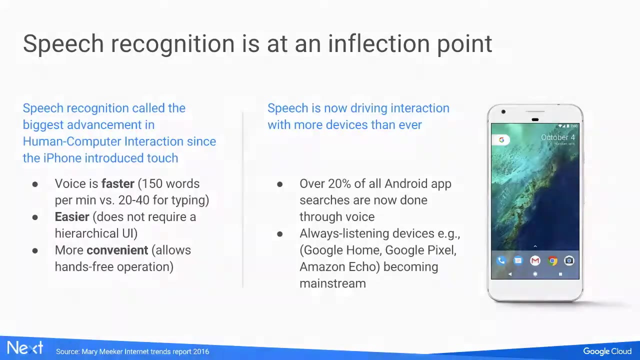 to this list, which is our new video intelligence API. So that's how speech sort of fits into the picture. We're very, very excited about speech. It's currently in beta. It's about to go GA very, very soon. So what is so exciting about speech? Speech recognition- People have been doing it for. 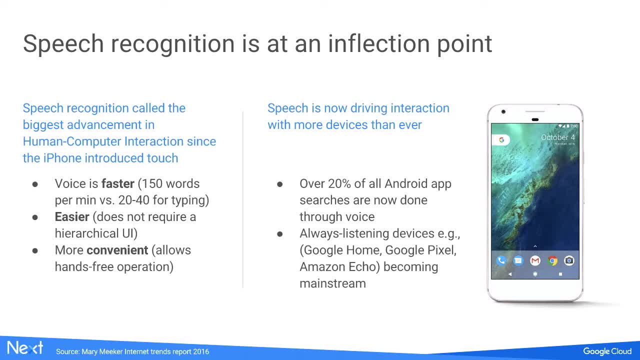 a very long period of time, But it's actually an inflection point right now. So other analysts have said It's a really great thing. It's a really great thing. It's a really great thing. It's a Yeah. it's now the biggest revolution in human-computer interactions since the iPhone introduced touch, so 10 years ago. 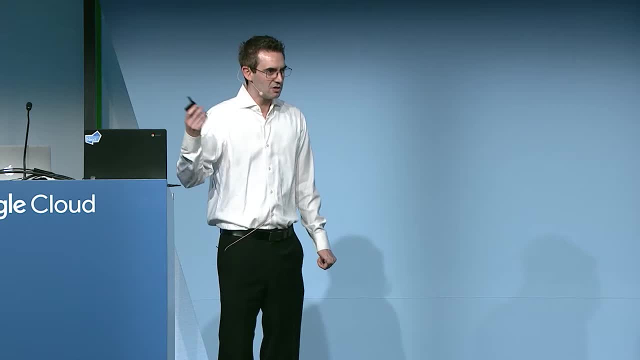 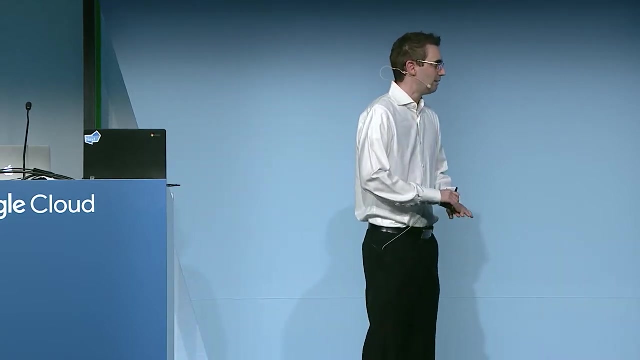 And you know it's dramatically changing the way applications are being developed and, you know, will be developed in the future. Voice is, you know, faster, easier, more convenient in many ways than typing or navigating through menus, And so we're seeing, you know, just in the last year, an explosion of voice apps, but in the future we're going to see even more of it. 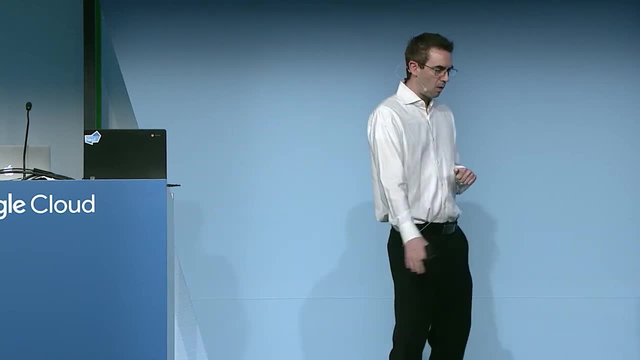 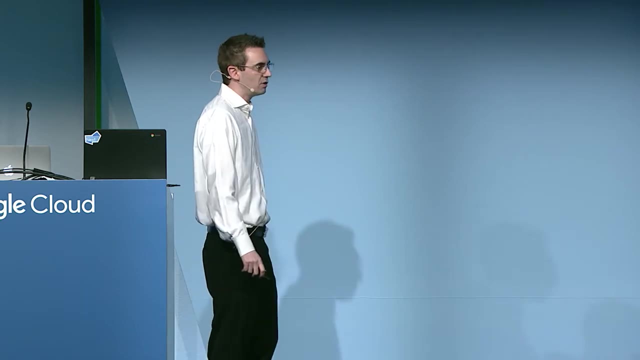 You know, today more than 20% of our Android app searches are already voice. you know, and we're very excited about that. We, you know, we want to make it as easy as possible to use all of our services. as you know, we're sure all app developers are out there. 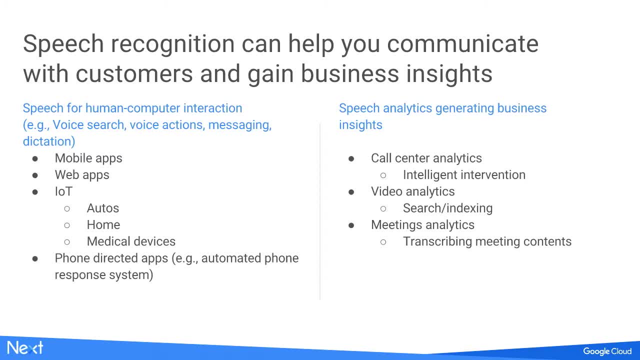 So in terms of the kind of broader landscape for speech recognition, you know what is it good for? We kind of see it in two broad themes. One is around human-computer interaction that we just talked about. so that is things like voice search, voice actions, messaging, dictation. 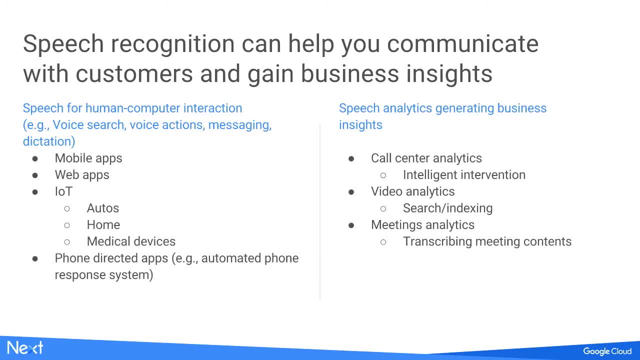 You know, this is fueling different services like mobile apps, web apps, connected devices and, to a lesser extent, also phone-directed apps, And basically enabling a new way for humans to interact with systems. The other kind of big domain is speech analytics. 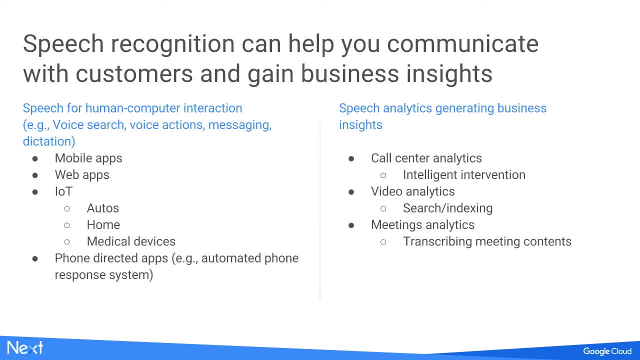 And this is fairly new. We're just starting to see this come out in a big way now because the technology is starting to be big enough, And that could be, you know, call center analytics, video analytics, messaging, meeting analytics- basically taking speech that is already happening in our world today and generating new insights from it. 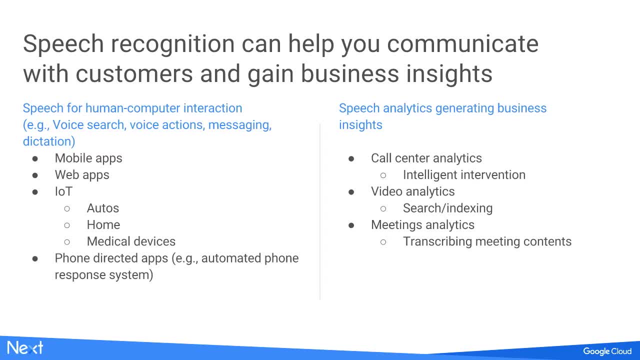 So I'm going to show you later a bunch of different demos more centered around the domain, on the left, on human-computer interaction, and I'm going to invite our guest speaker, Gary, who's going to show you how they implemented a very interesting use case on the right-hand side, on call center analytics. 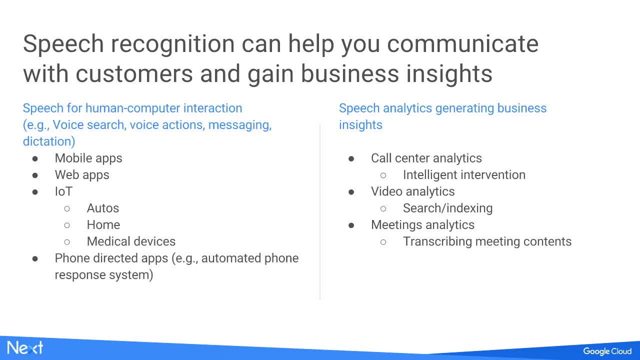 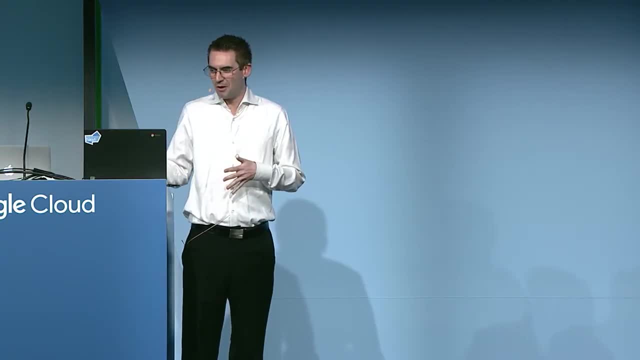 So you know it's going to be a fun session. We're also going to do a kind of a crazy code lab. I'm going to try, and you know, write an app in less than 10 minutes that will do speech recognition, sentiment analysis and translation using Google's APIs. 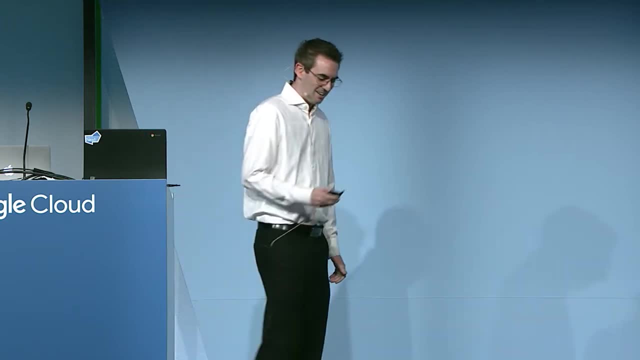 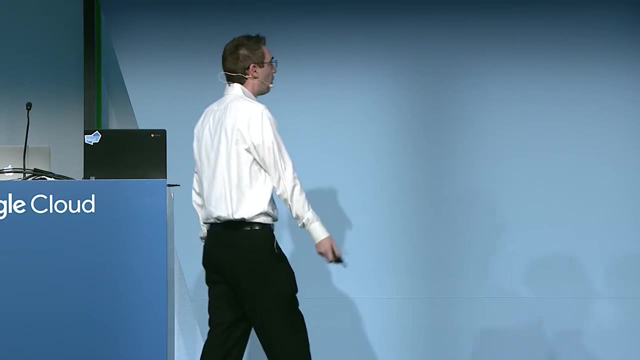 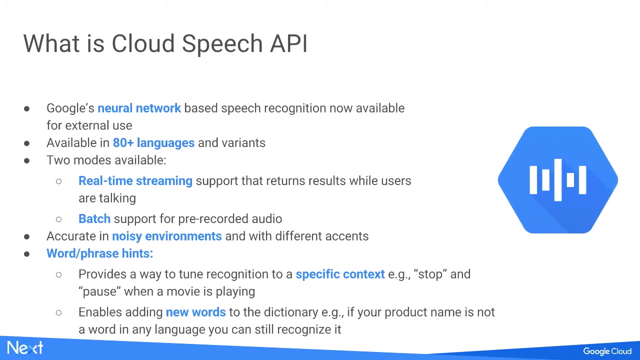 So hopefully it will work. We'll see, But we're going to do a little bit of that later, Okay, So you know what is Cloud Speech API and why are we so excited? So you know, it's our neural network-based speech recognition. 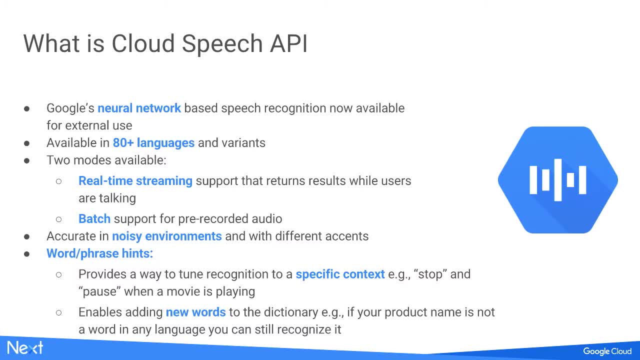 I already mentioned before, we're making it available for the first time now and it's universally available across 80-plus languages and variants. Basically, you know, I think more than half of the people that use smartphones today around the world are already covered, and we're aiming for more than that. 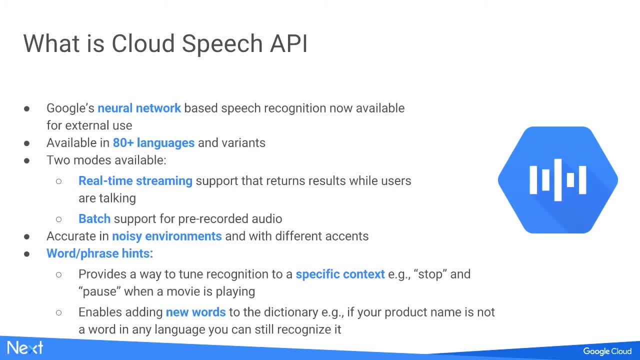 You can use it in two different modes- real-time streaming and batch- and I'm going to show you a little bit of both later today. And it's accurate in noisy environments and with different access. So when we built our speech recognition, we needed it to work, for, you know, people that are walking around in Times Square walking on with their phones and asking their friends to come in and talk to them. So when we built our speech recognition, we needed it to work, for you know people that are walking around in Times Square walking on with their phones and asking their friends to come in and talk to them. You can see the 1声 in the background gives you information about data below the screen. 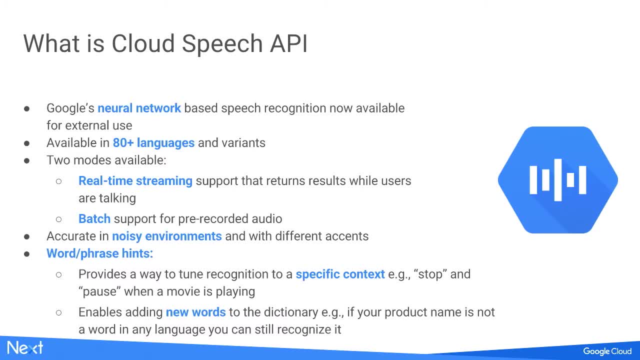 And you can see the 3声- probably tapes what's on their phone, what's the weather like in New York, while there's 100 other people right next to them, And so it knows how to filter background voices. But there's also people in India that are walking the street and there's a bus passing right next to them. 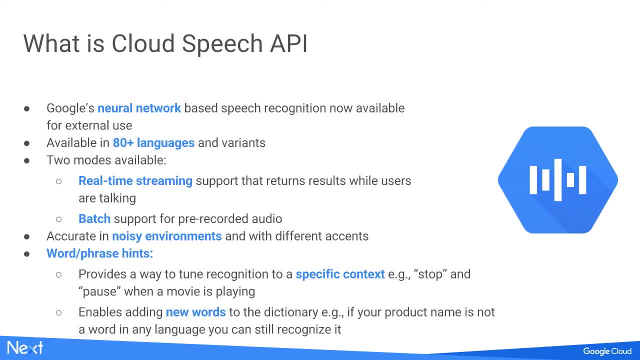 And so it knows how to filter kind of all different kinds of background noises and focus on the primary speaker. But there's also people in India that are walking the street and there's a bus passing right next to them. And the last thing here I wanted to emphasize: 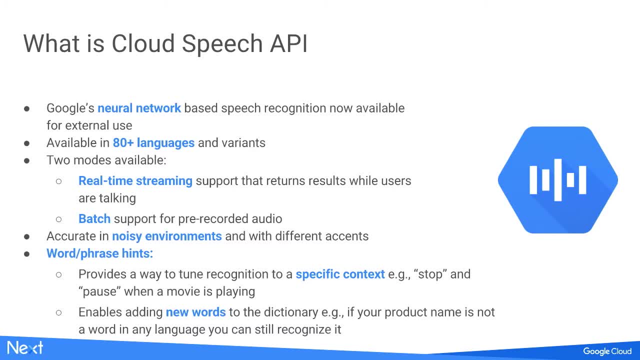 We have a really easy way of customizing speech recognition from Google. We can create our own voice여�. we don't handle those. We come in atartecom to export speech to your domain, so you know if you have a name of a company or a name of a. 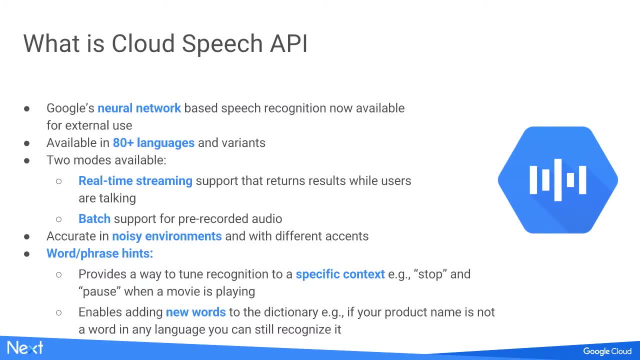 product. that's not actually a word in English or in the language that you're trying to work in. we make it really easy. all you need to do is just tell us what that word is and we automatically add it to the dictionary for you and we can. 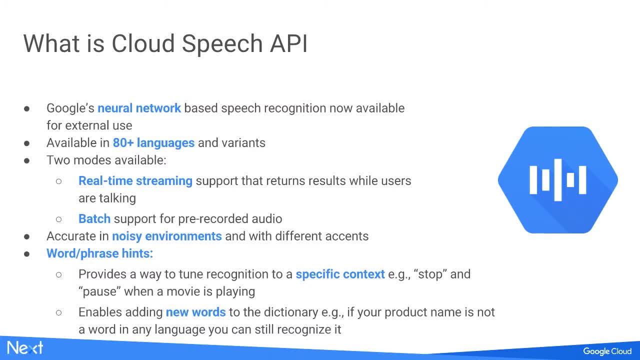 start recognizing it if you're in a specific mode in your application where you're expecting a certain command. so if you're building speech recognition for a player and you're playing a movie, so you might want to detect stop and pause, but then when you're not playing a movie, you might want to detect play or other words. 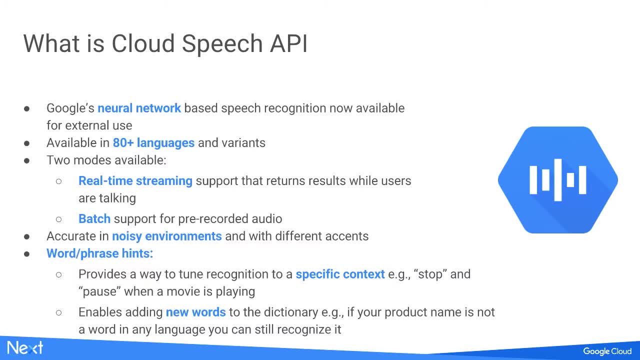 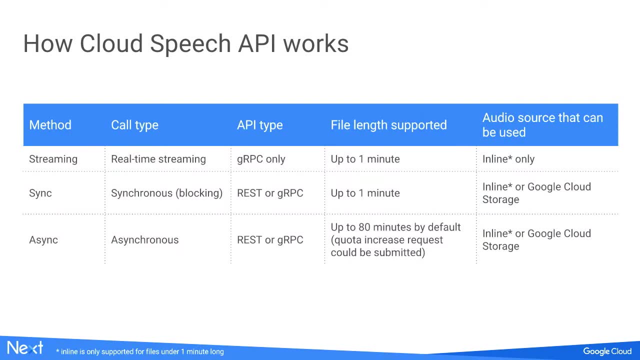 you can use word and phrase hints to detect exactly the words you need in the right context. so we have three different methods for using speech API: streaming, sync and async. streaming allows you to process speech in real time while the user is saying it, and so it's, it's, it's. 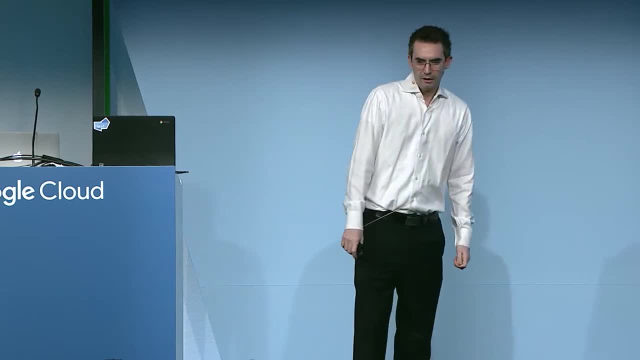 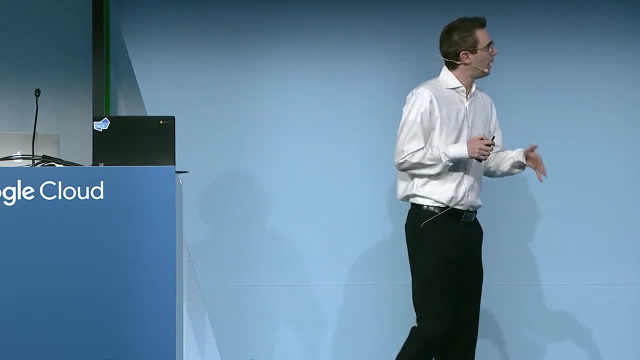 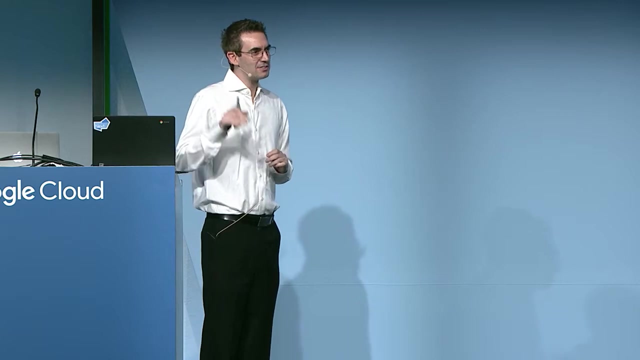 the fastest way of using speech API. it works with something called gRPC, which is our sort of improved binary version of rest, the gRPC. people are gonna kill me for saying that, but it's a. it's a. it's a faster, more efficient protocol and way of sort of accessing remote procedures. 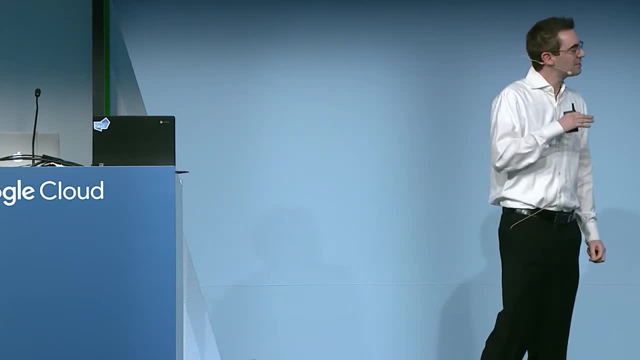 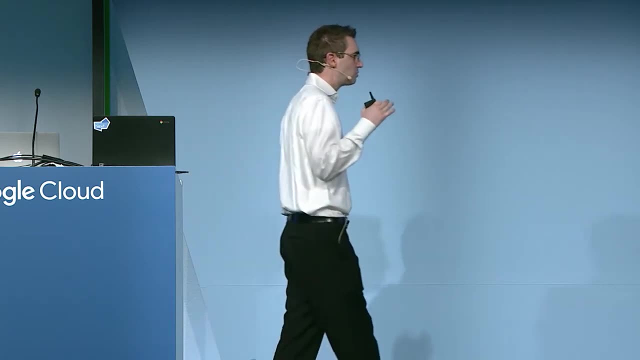 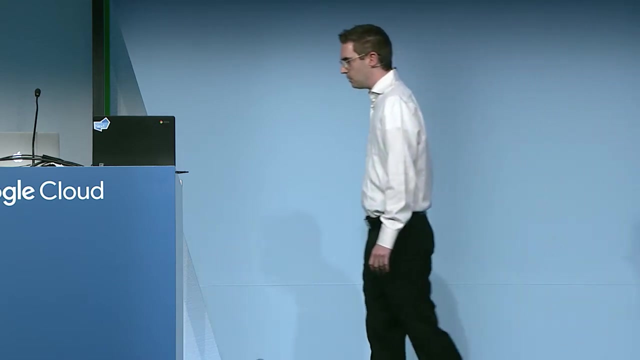 and allows you to process any audio up to a minute that's included in line in the request. sync is a much easier to use method. any you know it's a. you can use it on rest API. you can even do it with a curl command and it's it can process any. 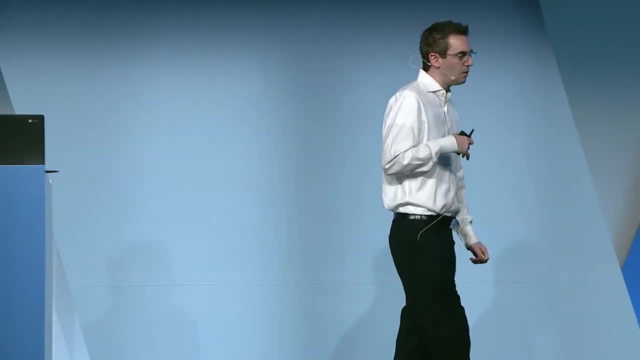 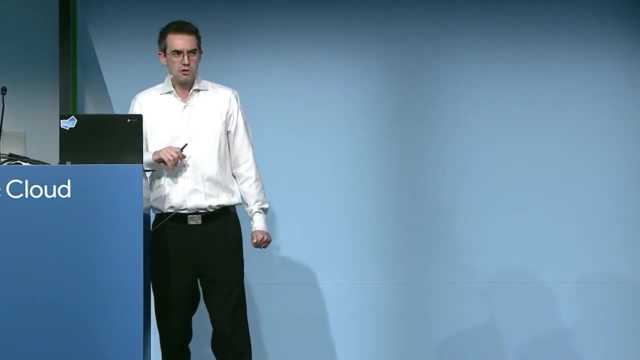 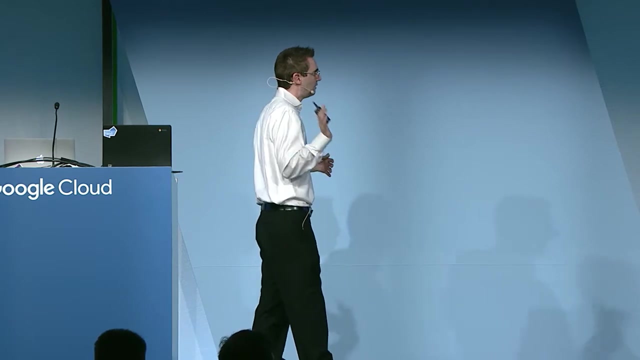 audio up to a minute. you can either embed the audio in line or use Google cloud storage and and then we have a sync which allows you to process larger files. it's basically not limited. it says up to 80 minutes, but you know that could be increased if you. 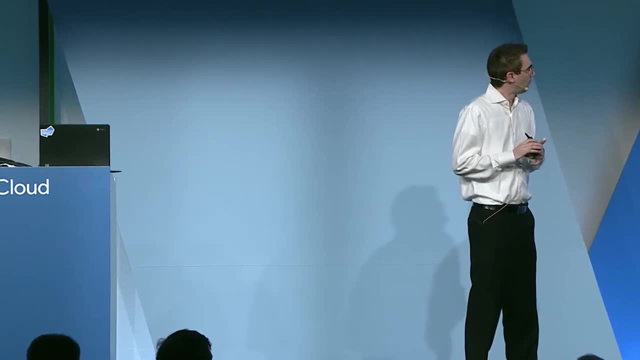 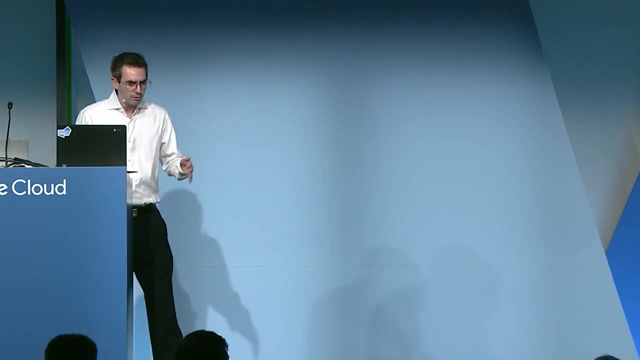 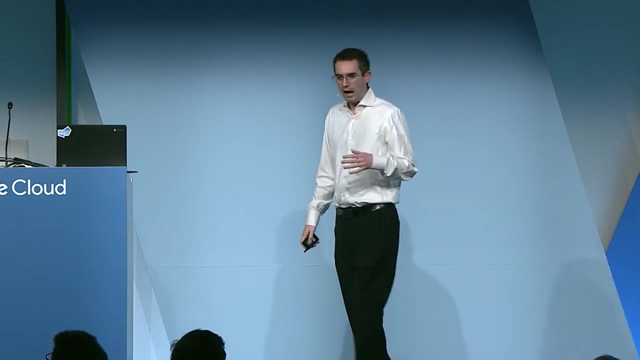 get a code increase and it can also be accessed by rest and process files either in line or a Google cloud storage. so with with a sync- because it's it's not blocking- you can quickly process a large number of files and process them in line or in line and then just check back in to see if they're, if they're done. 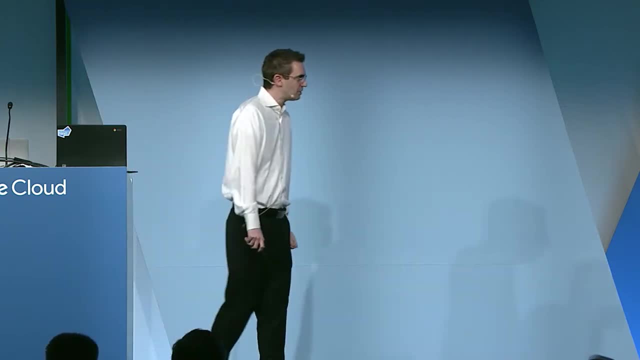 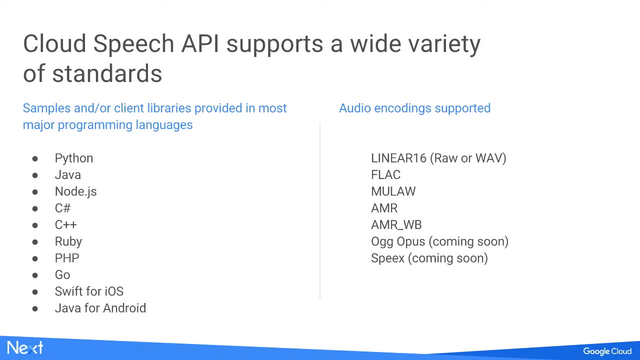 processing. in terms of standards, you know, when I wrote this- the slide I was- you know, even like I forgot, how many different standards we support. it's, it's, it's, it's pretty universal. that's something we're very proud of. you know, there's a large list of programming languages you can use to access cloud. 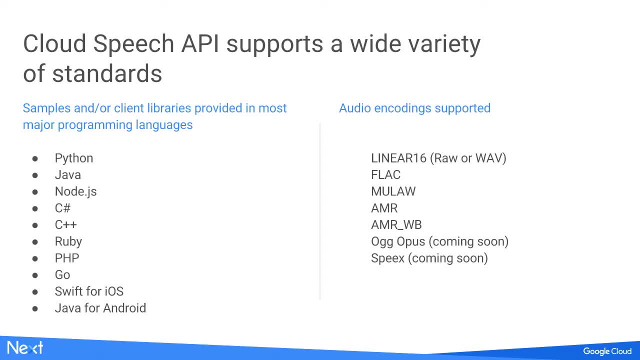 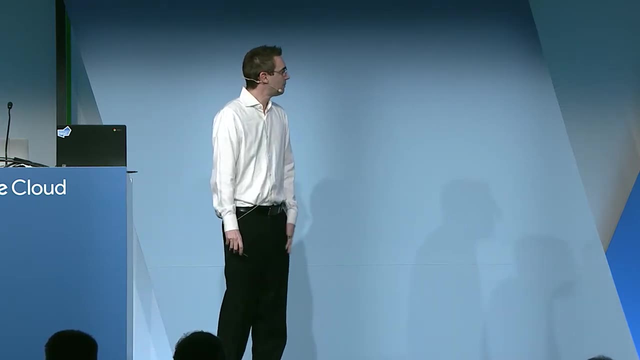 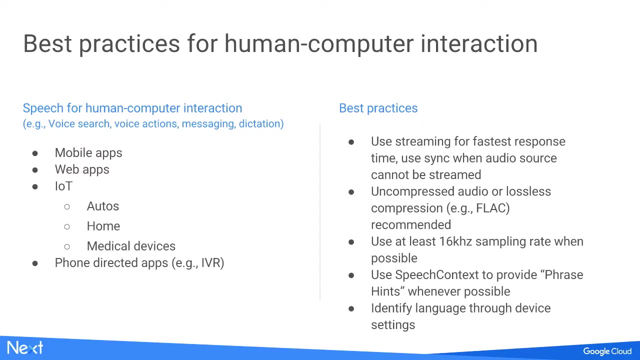 speech API and encodings that we support. Now, this is not an experimental project that someone at Google is running. This is a commercial service that we're fully backing and really developing, investing a lot in. So I wanted to give you guys just a little bit of best. 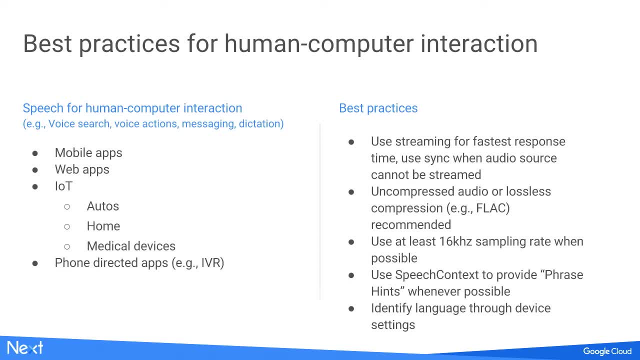 practices. if you are developing speech recognition apps, what would we recommend? And first slide is about human-computer interaction, so the left-hand side of the use cases that we spoke about earlier. So for human-computer interaction, you really want to use streaming whenever you can. 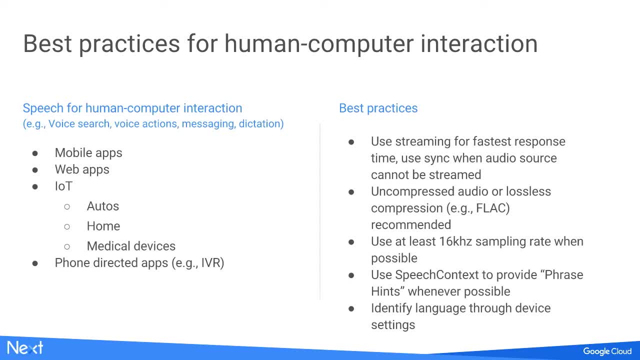 When you can't use streaming, you can use sync, But then there's going to be a delay and users are waiting for a response, So it's not recommended. You always want to use uncompressed audio if you can, And if you want to compress, you should. 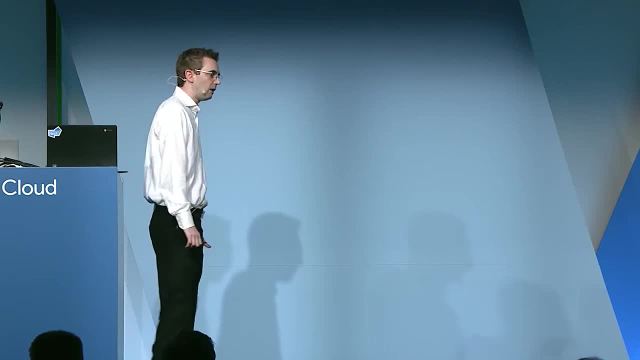 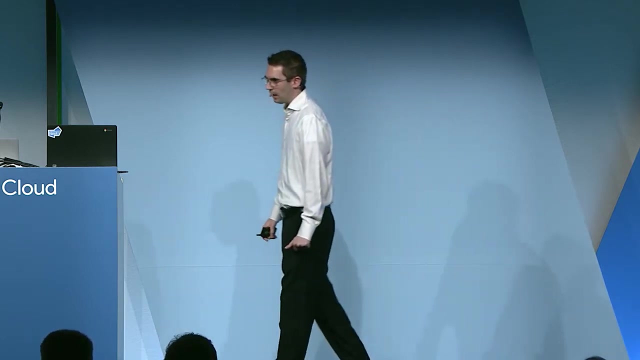 use lossless, Lossless compression, because lossy compression- like MP3s or things like that- they really degrade the accuracy of the recognition. Ideally you want to use as high of a sampling rate as you can, but at least above 16 kilohertz, or 16 kilohertz or more. 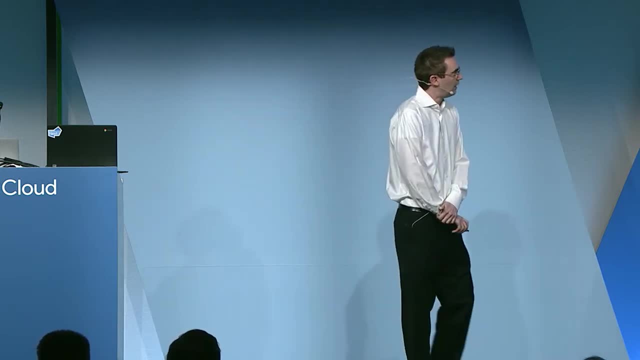 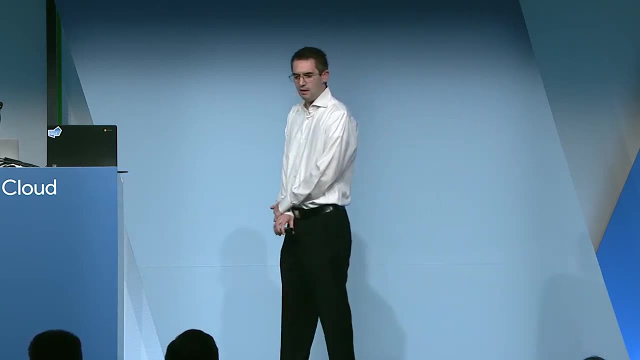 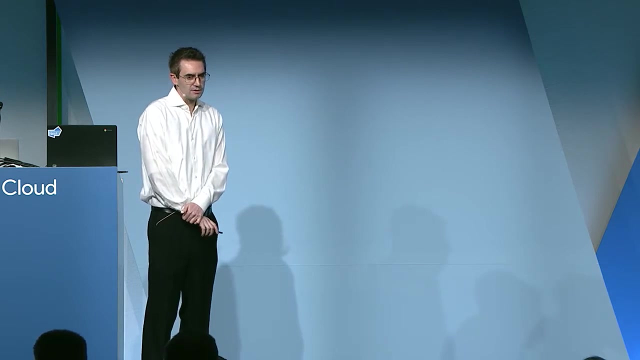 You don't want to go below that. if you want to use human-computer interaction, if you have a choice, if you're not running on phone lines, And whenever you can, you want to use speech context to get the best accuracy results that you can. 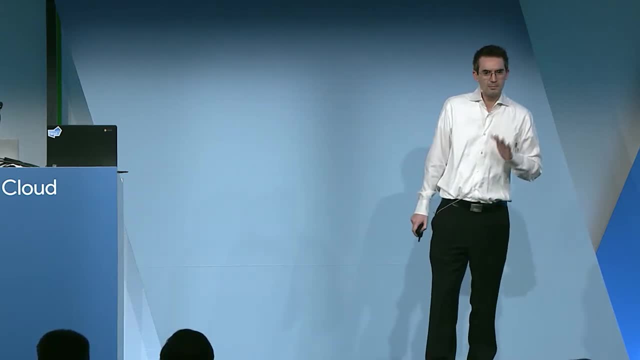 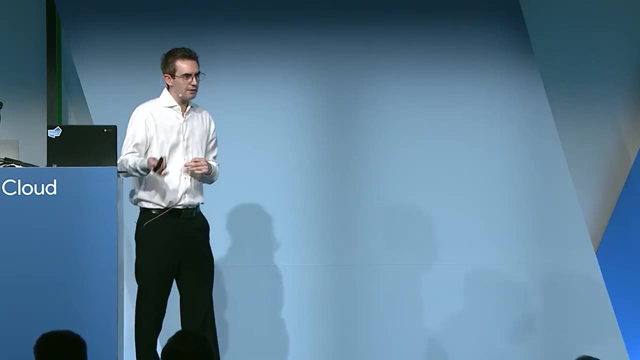 Now, using Speech API requires that you specify the language in advance. So what we see a lot of app developers do is they detect the language of the OS and that way they know what language the user is going to speak, And they provide that to Cloud Speech API. 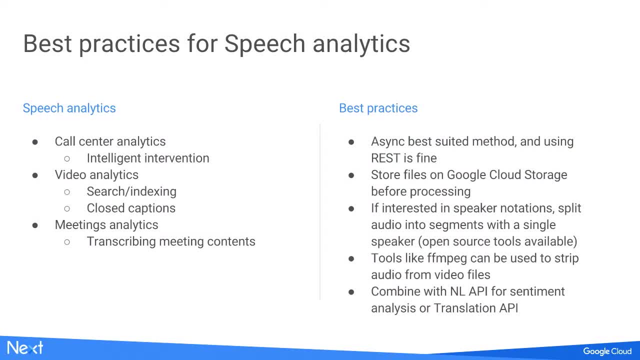 So then there's the other set of use cases, which are speech analytics. So there you're typically dealing with longer form audio, Like a call could be five minutes, 10 minutes, 15 minutes, A movie could be one hour, two hours, three hours. 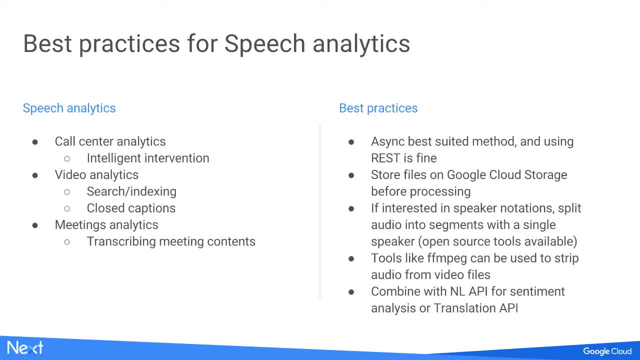 So you want to use async. most probably, You want to store those files on Google Cloud Storage and then process them in batch, And if there's multiple speakers, you may want to separate the streams so that you can process speakers separately. If you're processing a video, you 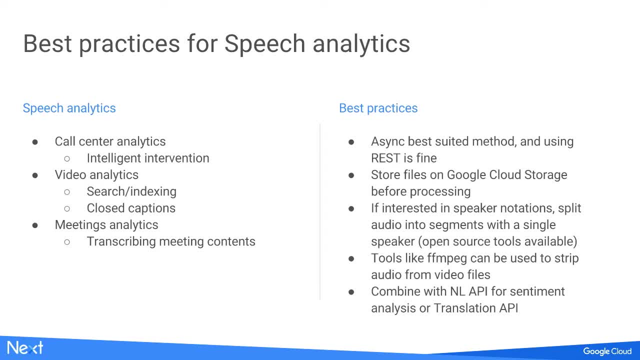 might want to use a tool like FFmpeg to strip out the audio and just send the audio to Cloud Speech API And it's very easy to combine it with Natural Language API and Translation API, which you're going to see In a second. 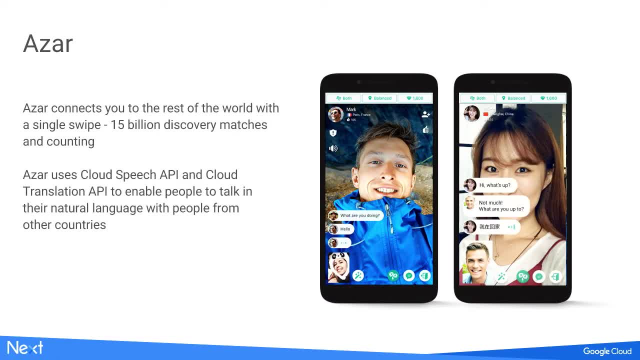 OK, I wanted to give you guys a few examples of human computer interaction, because we're going to spend more time later about speech analytics. So Azar is a video chat discovery app. Does anyone here in this room know about Azar? OK, a few. 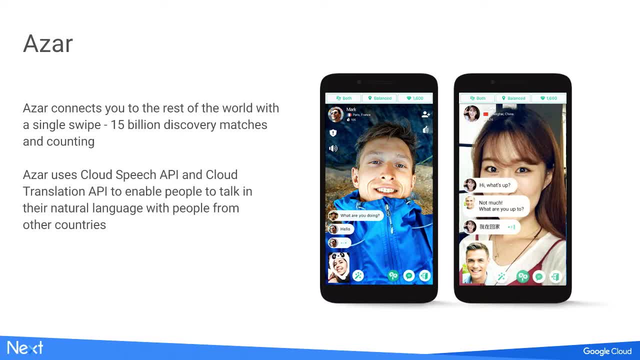 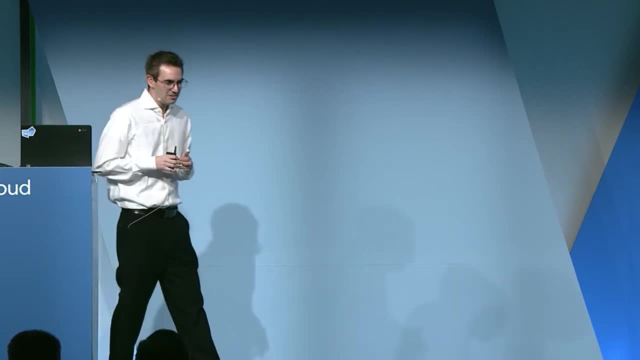 So apparently they have 15 billion discovery matches already. So what they do is they connect people with new people that they don't know, And they've done it 15 billion times already. Every time I hear about this, I'm just shocked. 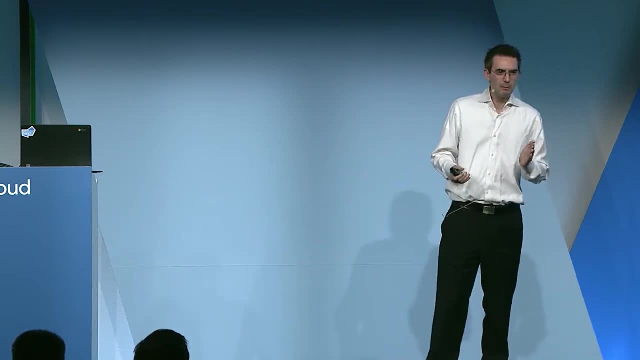 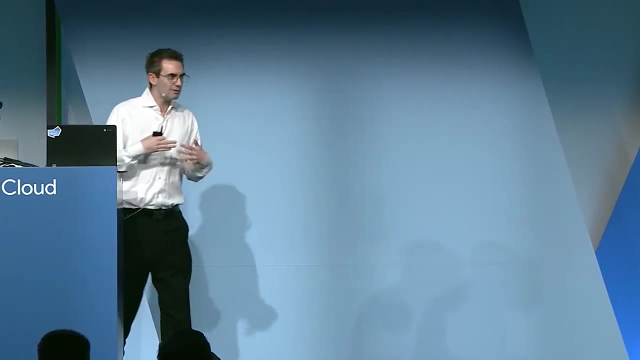 And most of the time, or many times, it's people in different countries that speak different languages And there's a little bit of a language barrier, Like you could imagine. Imagine when two people from different countries want to talk to each other. 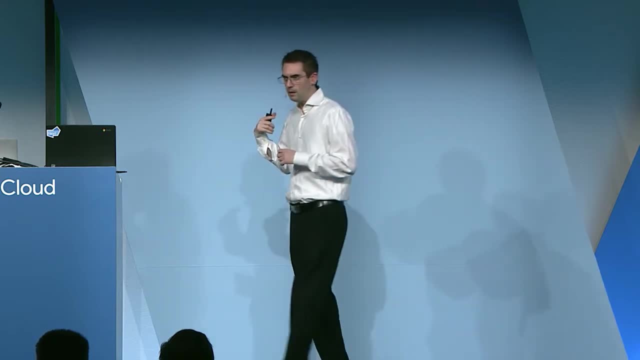 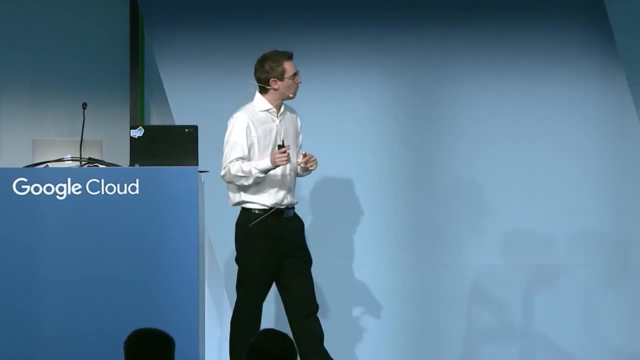 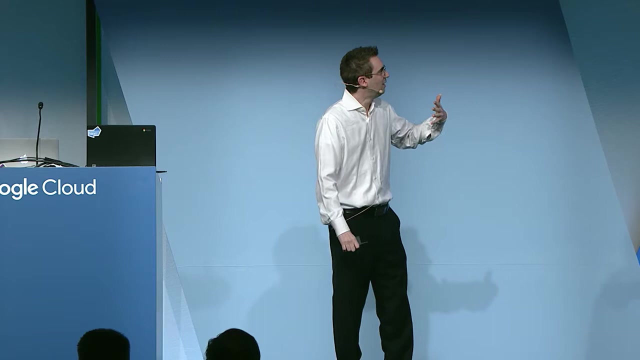 So what they do is they use Cloud Speech API to transcribe the speech into text And then they use Translation API to convert that from one language to another And they allow two people in different countries to talk to each other. And as they're talking, they see on the screen. 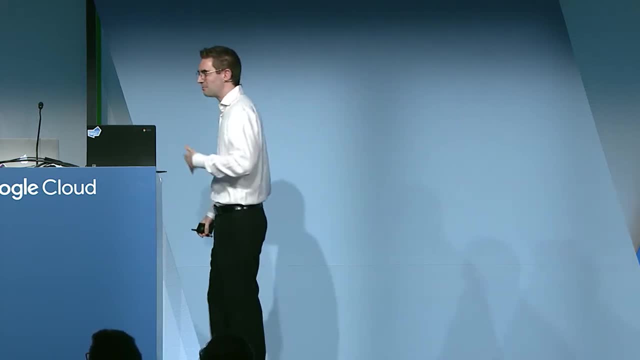 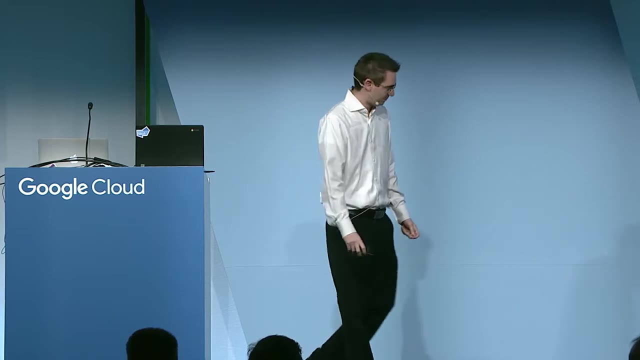 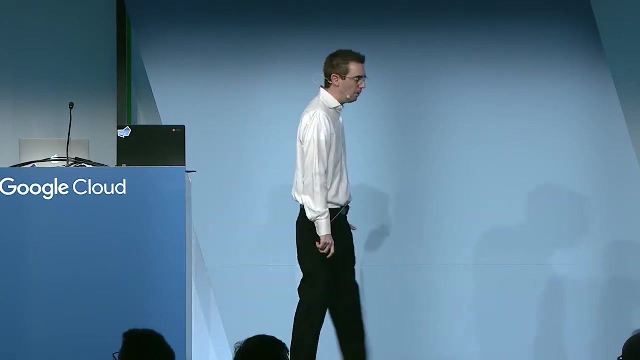 what the other person is saying And they can react to that. So it's pretty cool. It's really sort of enabling use cases that were not really possible, Maybe even like one or two years ago. Very, very exciting. Another example is Tribe, which is a messaging app. 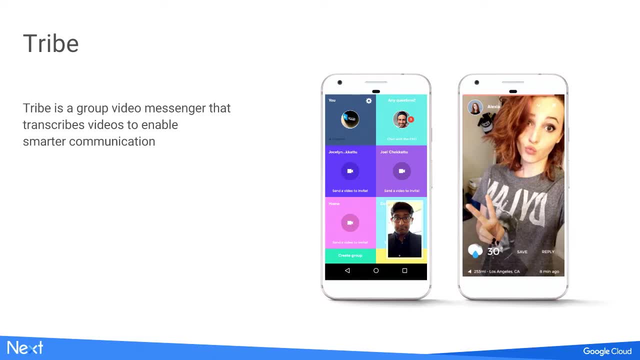 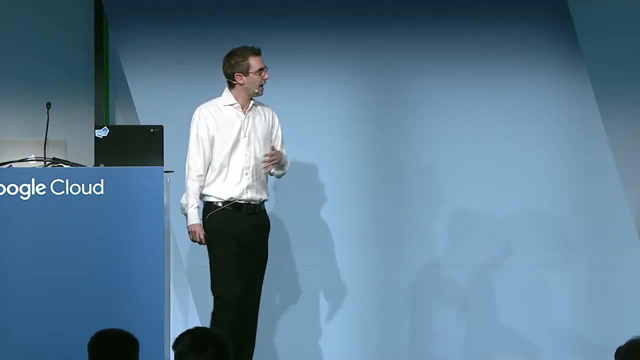 that uses video And it allows people that don't want to type a message, They just want to say something to their friends. They can record a quick video, say whatever they want to say And Tribe will show the video. enable adding text to that video by transcribing the text. 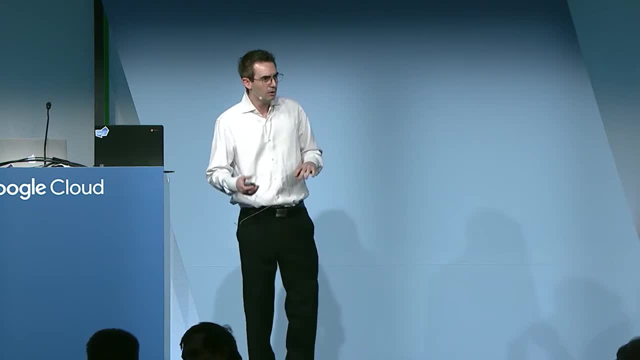 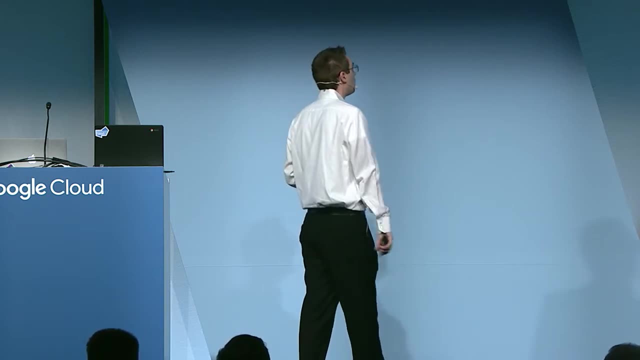 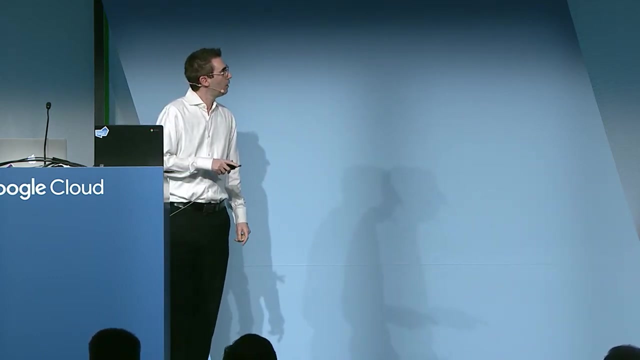 and defining some sort of keywords or alerts or things like that. So if you mention a dinner or a restaurant or something, it can sort of react to that and give the user more information about what they're talking about. Pretty cool, OK. So now I want to show you guys a few demos. 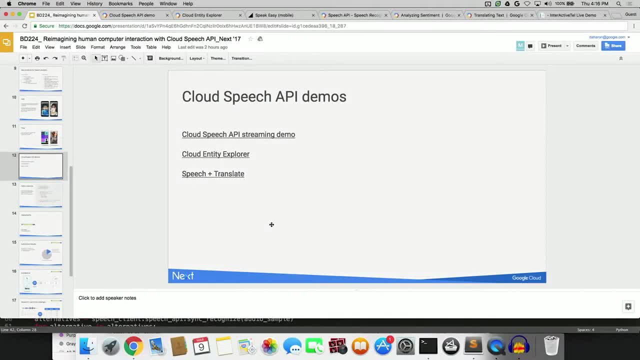 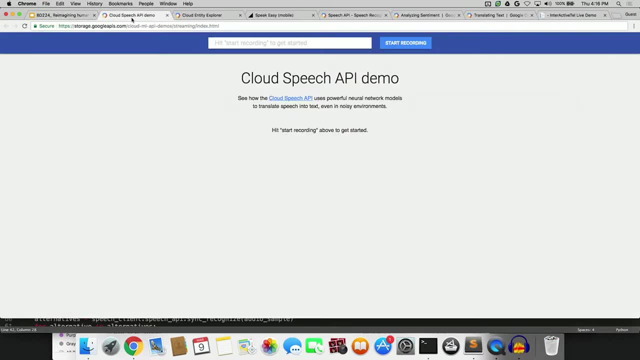 Can we switch to the demo computer? Yeah, Cool. So this is always risky. Speech recognition demos in a large room with Echo is not what it was intended for, But what I'm going to show you now I'm just using a regular computer. 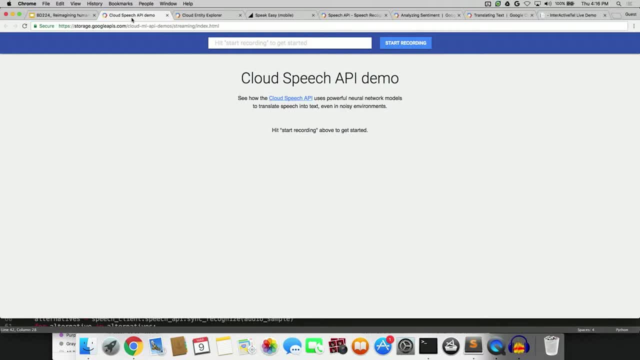 And I'm using the mic from my computer. Nothing special, no special equipment. I'm just going to talk close to the computer And let's see what it's able to do. So OK, that passed by. OK, I think it got 100%. 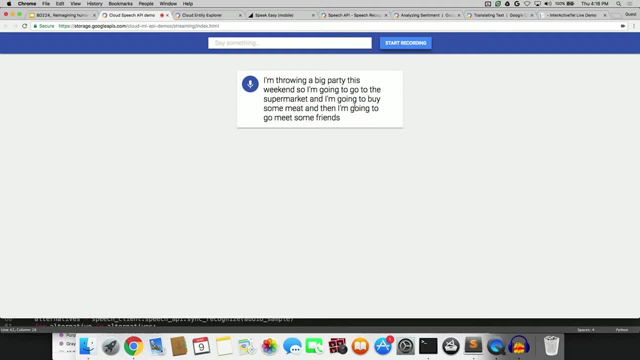 I'm not sure. Usually it gets 100% or close to it. It doesn't always get every single word, But I think this time it might have. And I don't know if you guys noticed, but while I was talking you could see on the top. 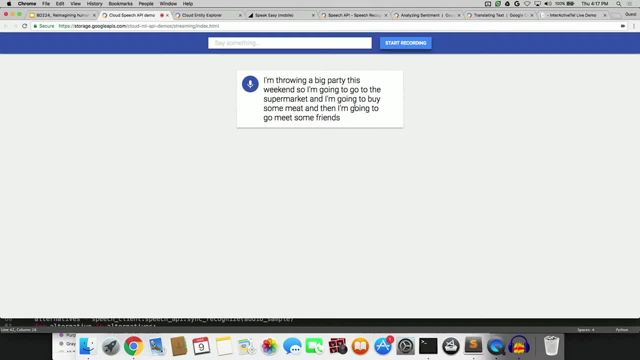 the words were appearing in real time almost in the exact same moment that I said the word. So it's pretty impressive. It's very, very fast. The other thing I would say is interesting here is you can see that I said the word meet twice. 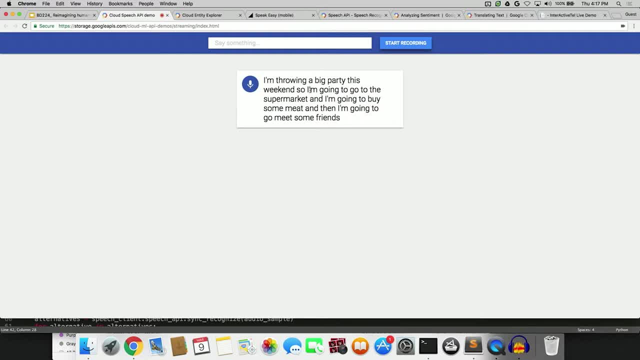 And even though I pronounced it in exactly the same way, it knows how to differentiate And from the context of the sentence, it knows when I said this meet and when I said that meet. So every time this works, I'm always amazed. 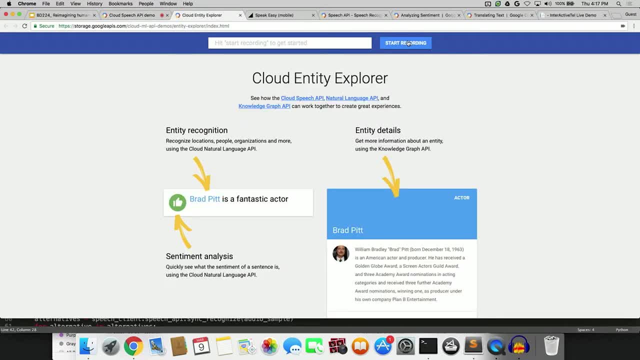 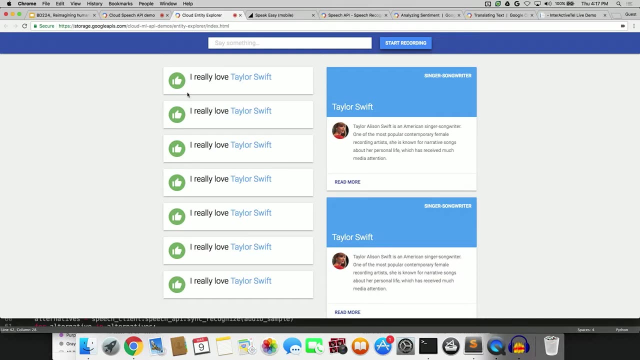 It's pretty cool. Let me show you something else. I really love Taylor Swift, which is true, by the way. OK, we have a bug in the demo here, But you can see this demo uses a couple different elements. So one is it combines Speech API with Natural Language API. 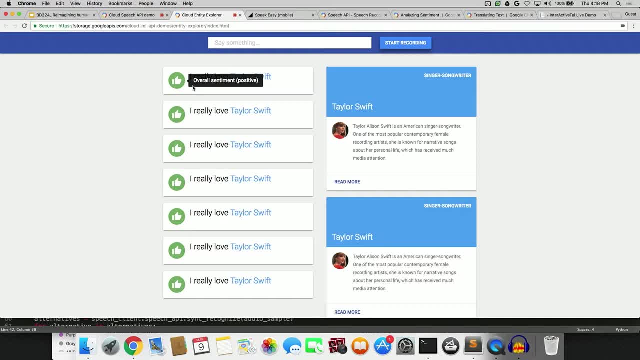 So you can see the overall sentiment is positive. So it detected that And it also extracted the entity Taylor Swift And it brought up a card. It knows it's a singer-songwriter. It has a little bit of a description from Wikipedia. 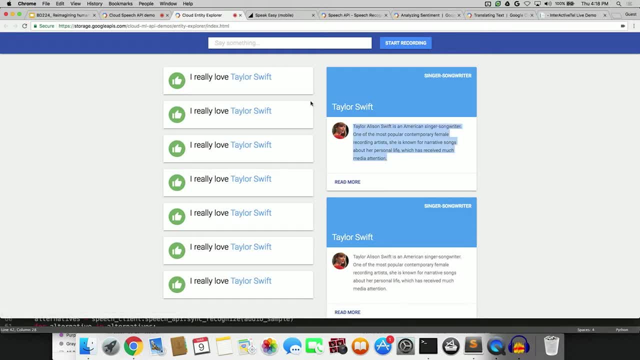 And you can click on the link. But the other thing I wanted to show you is our speech recognition was built originally for our search engine, And so it's built to recognize named entities really, really well. You know, You get searches for every single entity you could imagine. 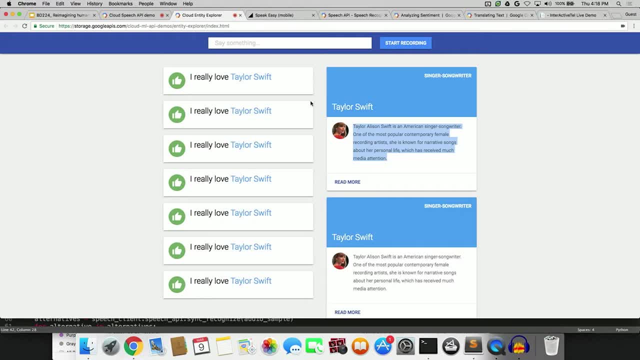 And a lot of those searches are voice searches, And so we developed our speech recognition in a way that it knows how to handle that, And when you mention entities with speech, we will detect them even if it's not a word in English. 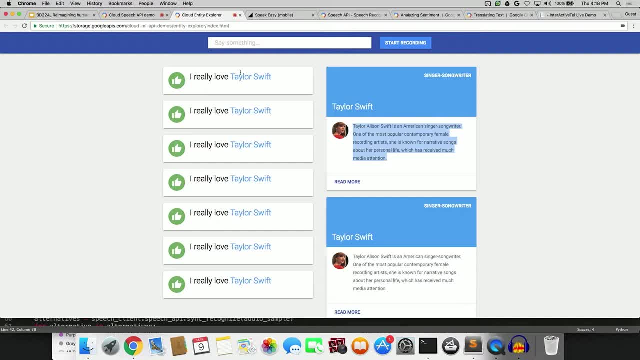 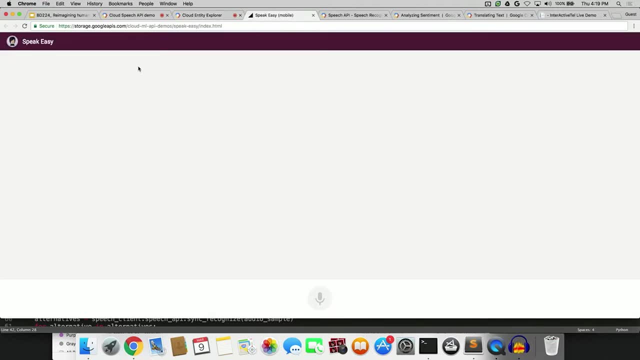 And we will format them so you can see it's capitalized And it knows how to recognize the entity. So the third and last demo. So this is a demo. This is a demo that sort of tries to teach you how to speak a new language with speech API and with translation API. 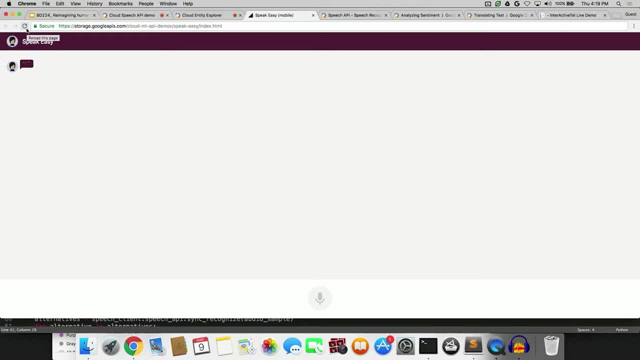 So it's going to detect that I'm in an airport and about to fly to Tokyo And it's going to try and teach me Japanese. Did you guys hear that Konnichiwa? OK, It wants me to say konnichiwa. 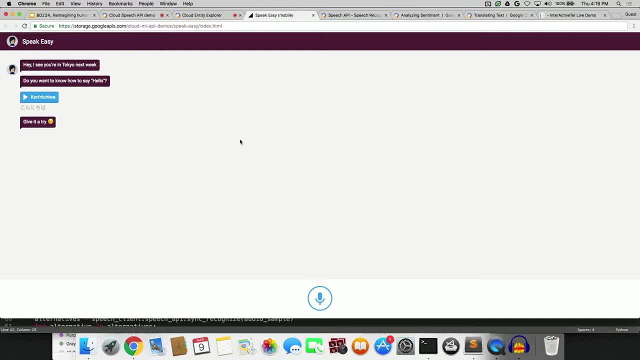 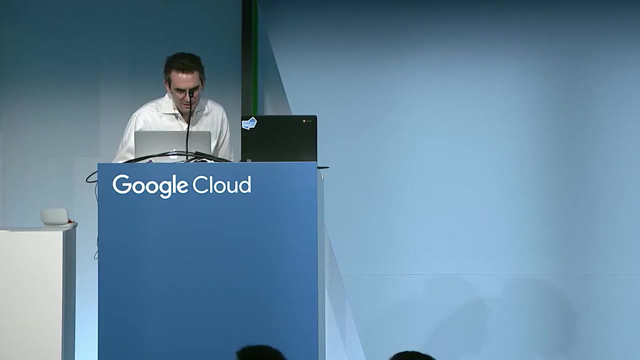 So I'll try and get this wrong: Konnichiwa, Konnichiwa, And let's see what happens. Konnichiwa, Konnichiwa. OK, That wasn't wrong enough, Let me try this one: Ogenkisaka. 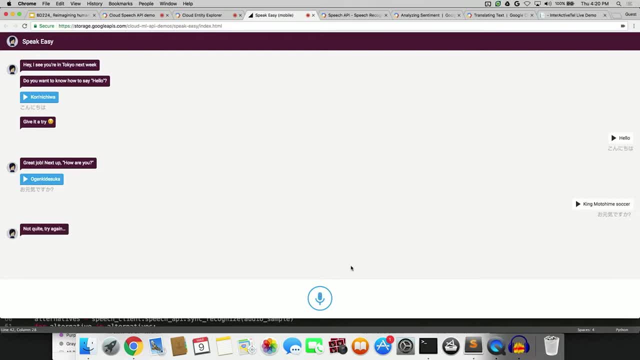 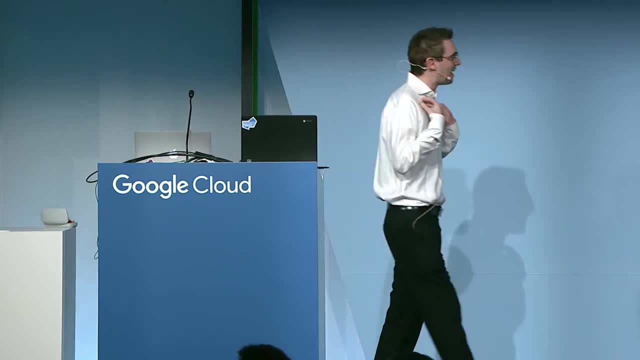 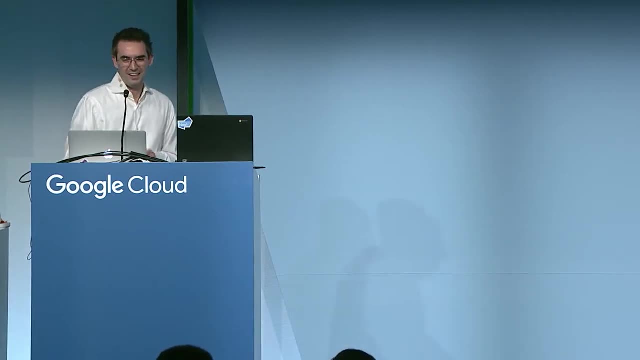 Ogenkisaka, Ogenkisaka. So apparently what I said in Japanese is King Motohime Sokka. So it actually recognized my language in Japanese and then translated it back into English. So pretty cool, OK. So these are sort of pre-prepared demos. 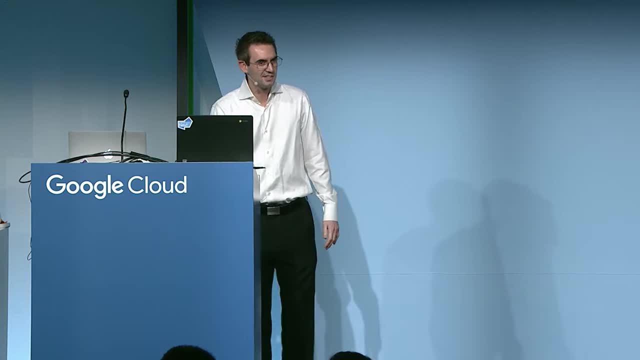 And you'll say: OK, that's fine, But how easy is it really to use? So what I'm going to show you guys, if you just go to the app, you can see the demo. You can see the demo. You can see the demo. 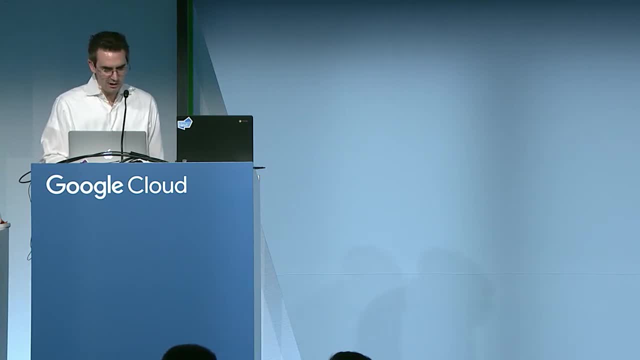 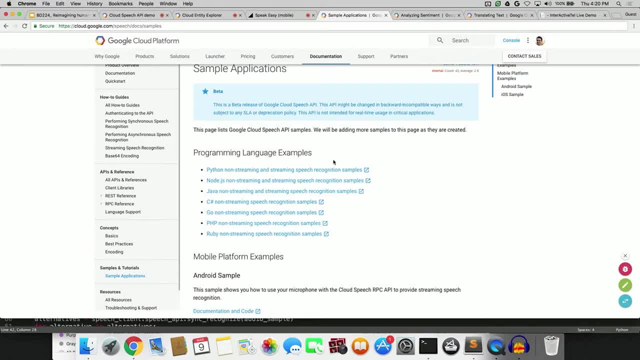 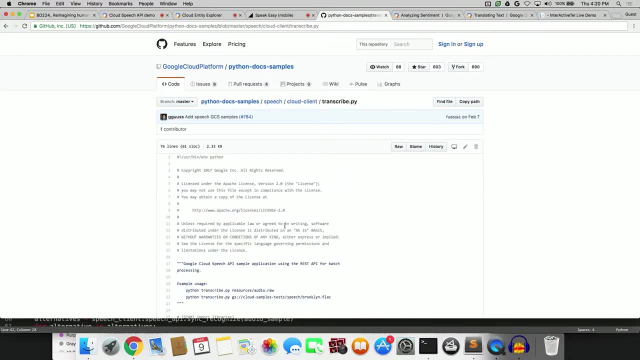 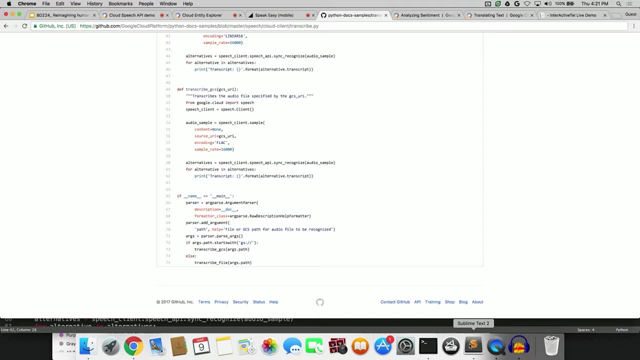 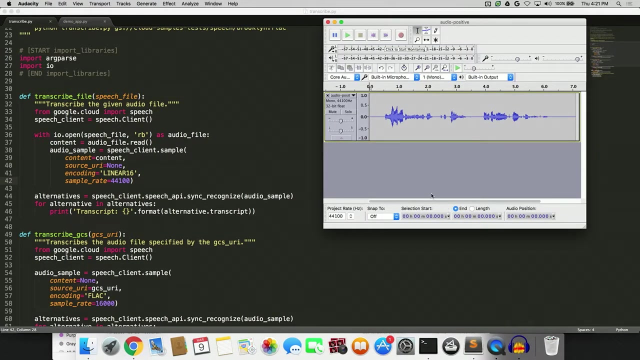 You can see samples for all the languages that I mentioned earlier. I'm going to go to the Python sample And you can see there's basically a Python example here And I've loaded it onto my PC And I pre-recorded this audio file. 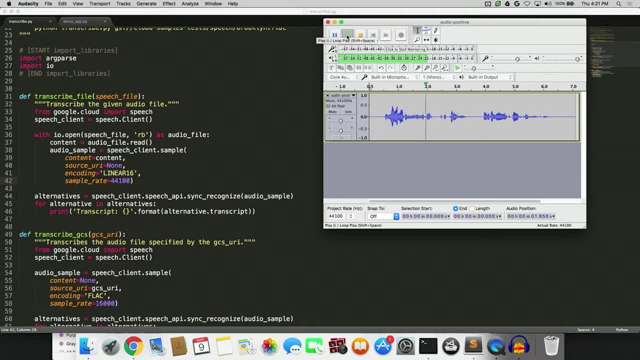 I'll play it for you guys. I'm really loving this session so far. It's pretty awesome. I especially like all the code examples, So hopefully that's representative of some of you. If not, then maybe a little bit later. 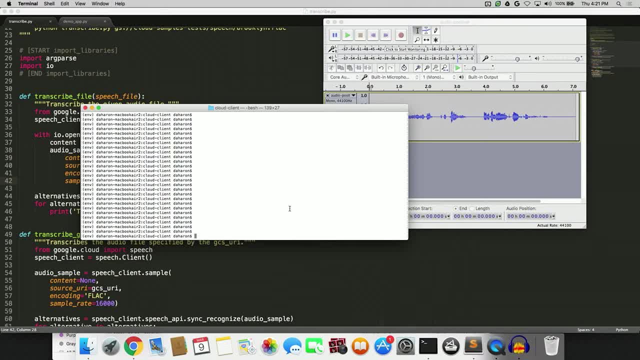 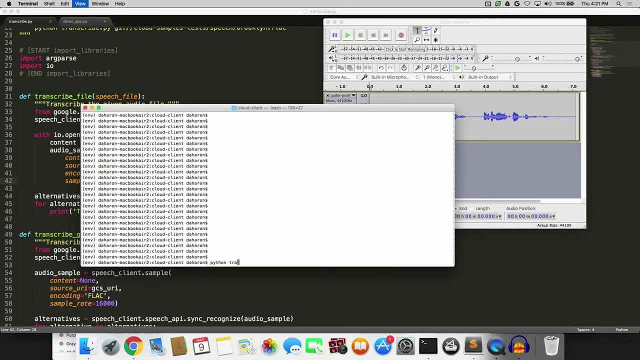 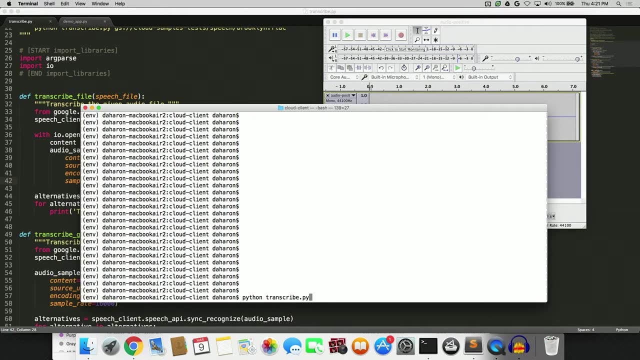 And let's try- and you know I pre-downloaded this demo, Let's try. Can you guys see my terminal? Maybe make it bigger, Better now, OK, I'm going to try and transcribe it And let's see what's happening. 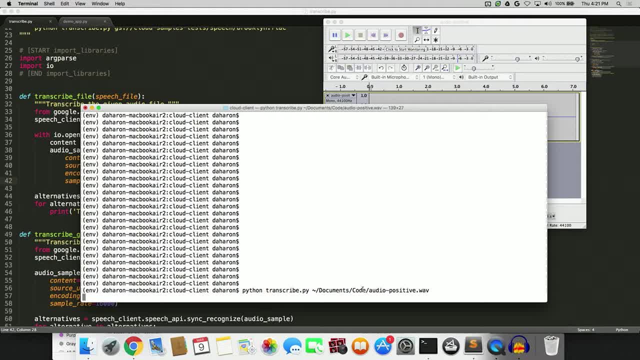 So it's taking this file that I recorded in a library called Code And it's sending it to the cloud and getting a result back. So you can see I'm really loving the session so far. It's pretty awesome. I especially like all the code examples. 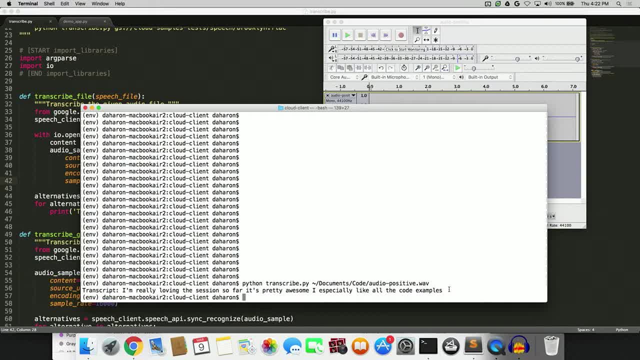 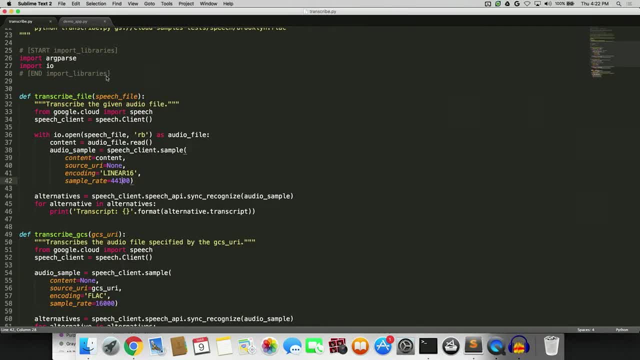 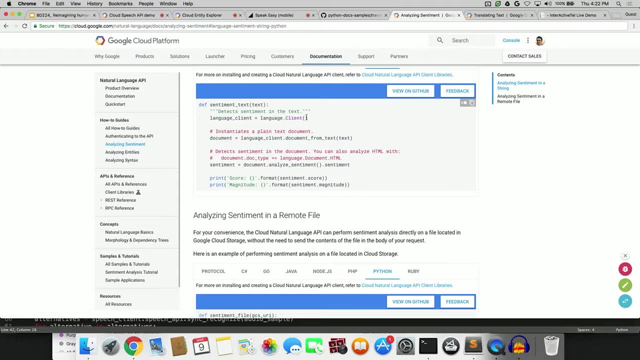 So it kind of got the gist of it. But now you know what happens. Let's say we wanted to add sentiment analysis to that. How do we do that? So I'm going to go to our Natural Language page And if you just click, How to Analyze Sentiment, 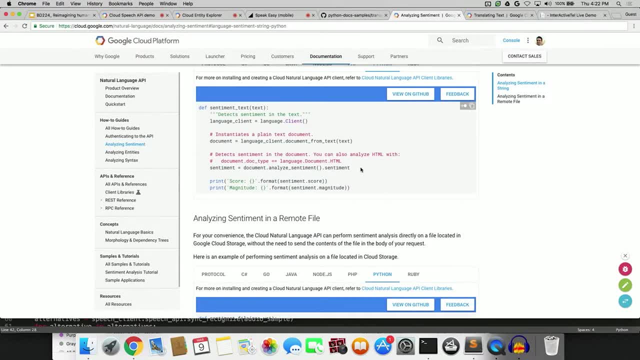 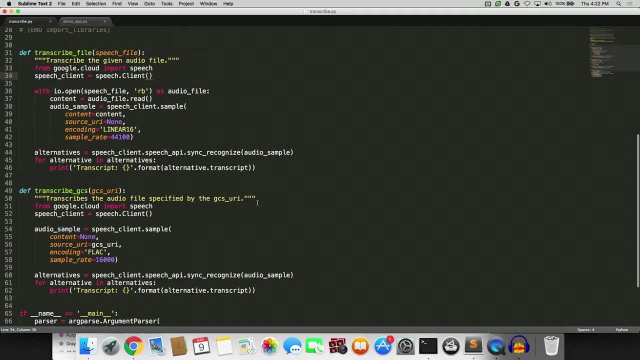 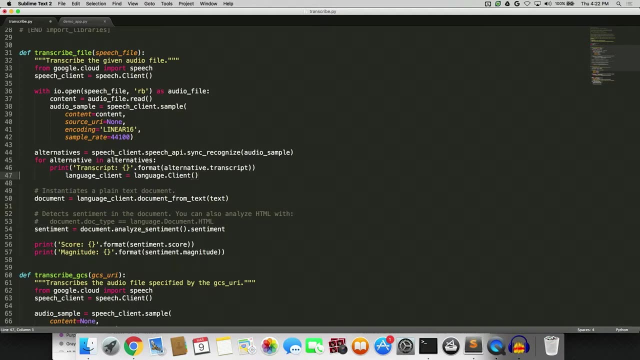 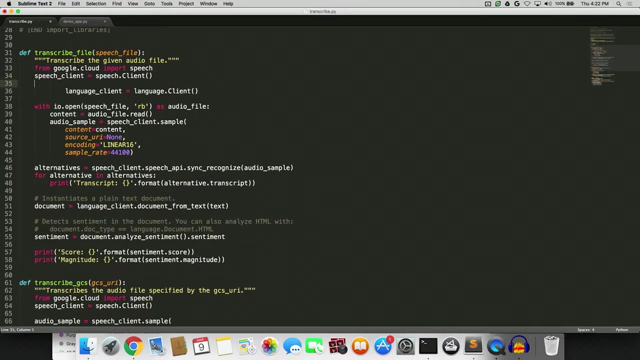 and go to Python. there's a code segment here, So I'm just going to copy it and add it here to our Python script And I can just put this up front here And let's also import from googlecloud import language. Let me fix the indentation. 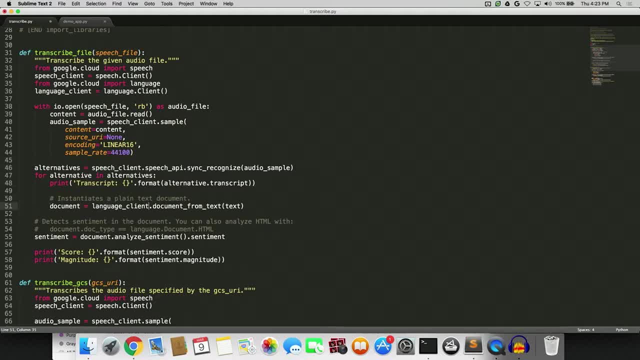 And now we want to feed it this text alternativetranscript, which is what comes back from the speech API. So let's feed that here And then we do the sentiment analysis And then let's print this And the sentiment score. I don't think we need the magnitude. 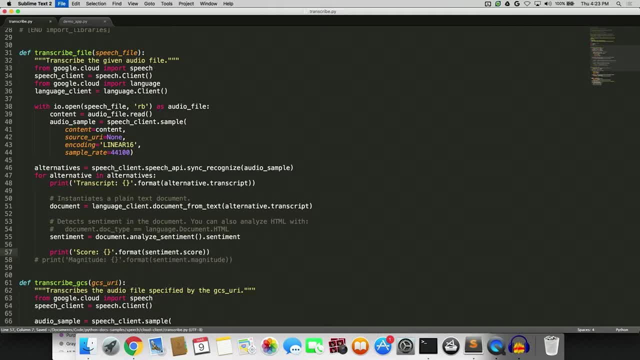 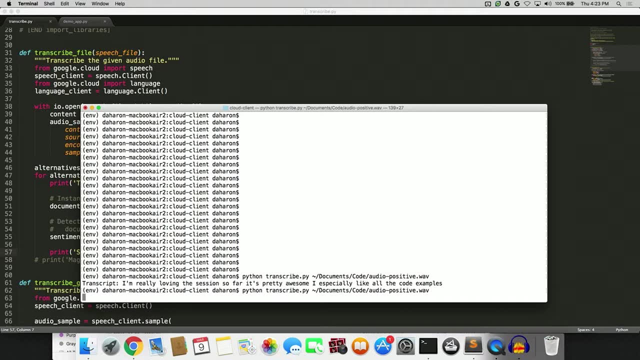 So we can just hide that. Let me save, Let's run it and let's see if it actually works. So this is OK. So it worked. It got the transcript And it got the sentiment score. So what do you guys think about that? 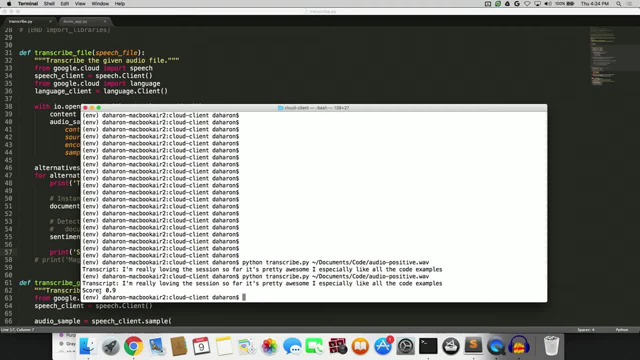 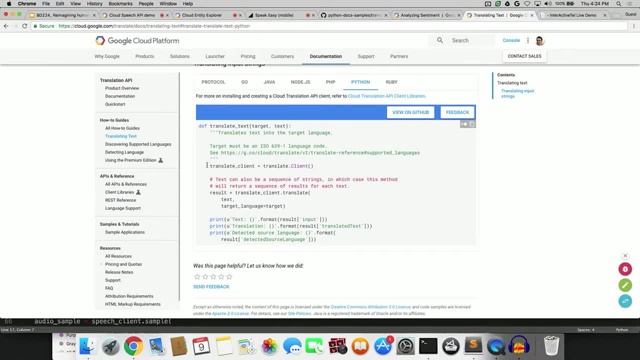 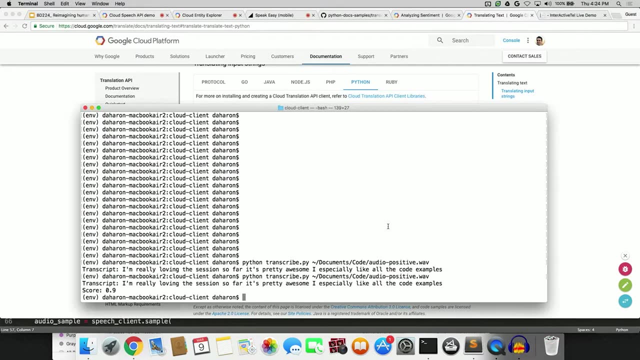 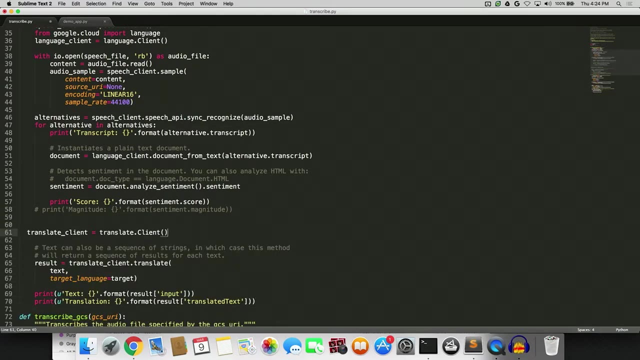 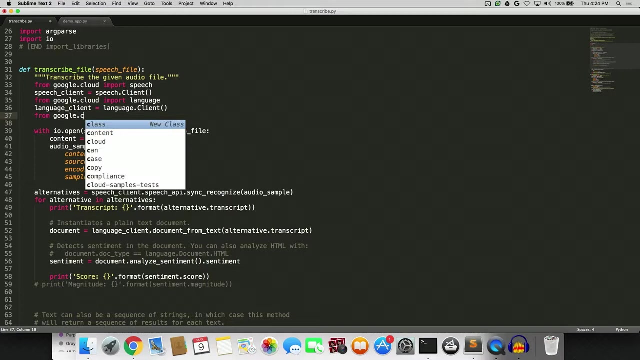 That was pretty easy, Okay. so let's make it more complicated now and let's also add translation, and let's go back to my editor and let's paste it in here. I'll put the client up front and I'll import the library from googlecloud. import translate. 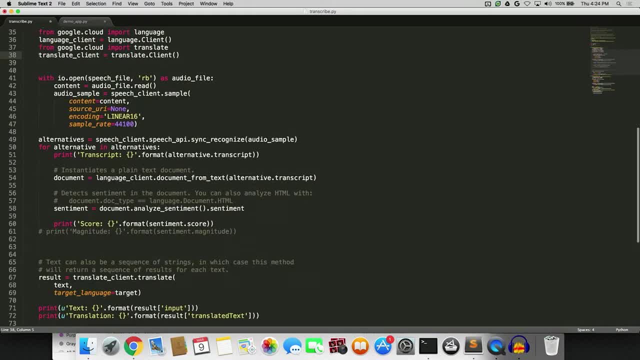 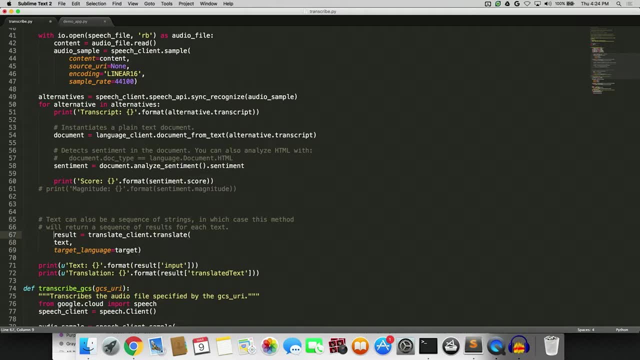 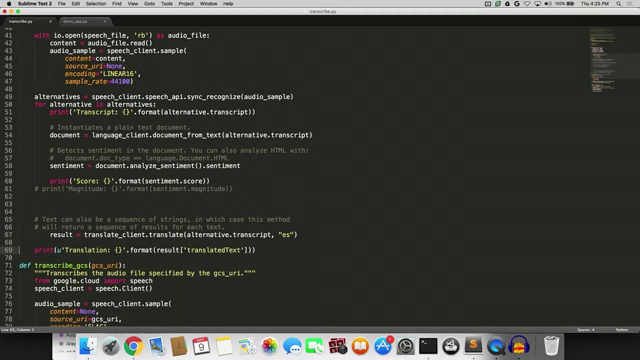 and let's add this here and now. let's feed it. instead of text, let's give it this alternative dot transcript: Okay. And instead of target language, let's just give it ES for Spanish. and now we don't really need the text because we already printed it. 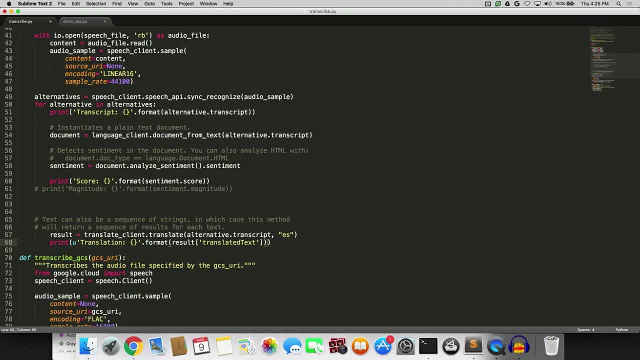 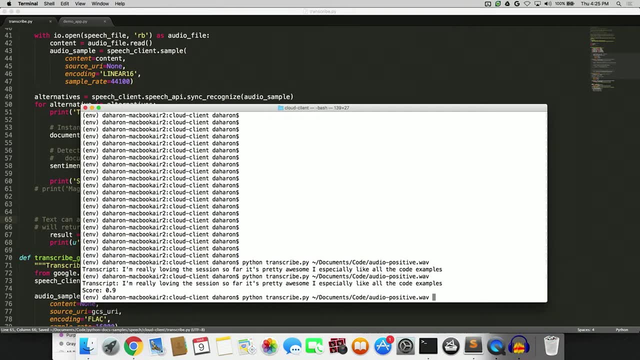 Let's print the translation. Okay, Now let's run it. let's see what happens now when we run it with the combination of text. So what it should be doing now is showing us the transcript, then showing the score, and then showing the translation. 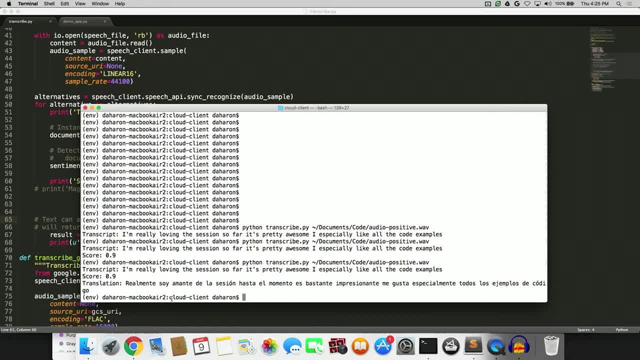 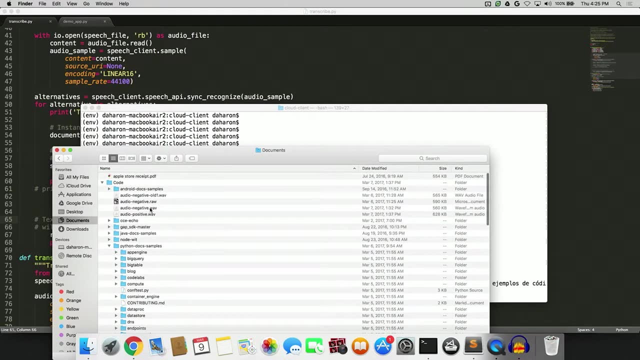 So that's it, We have it. It worked in Spanish and with sentiment analysis. Let's try one more thing. So I wasn't sure if you guys would really like this, so I also recorded a different option. Okay, Let's see. 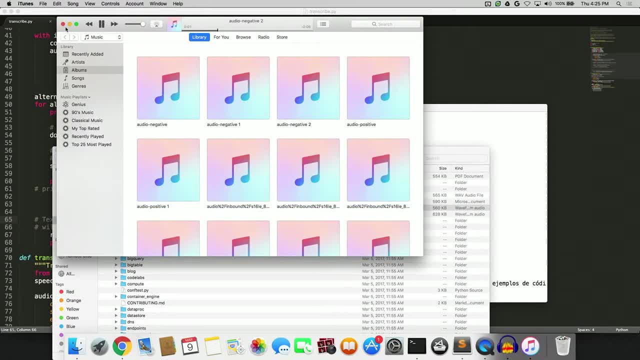 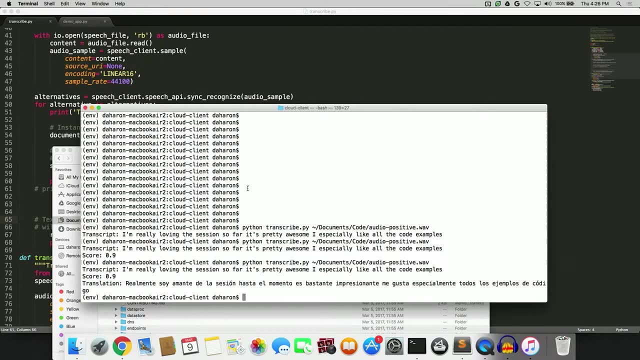 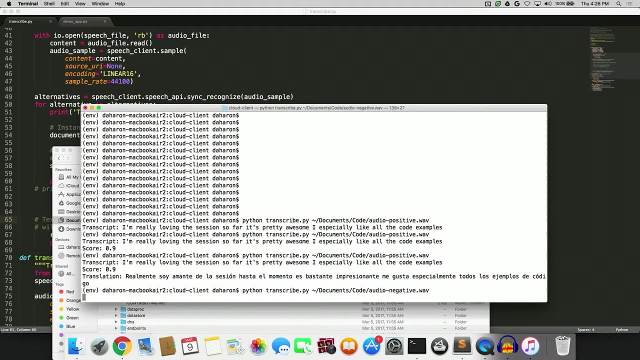 Okay, Let's play it. Let's play it. I really hate this session so far. It's very boring. I can't wait until it's over. Okay, So let's try and transcribe that with speech recognition and also analyze sentiment and 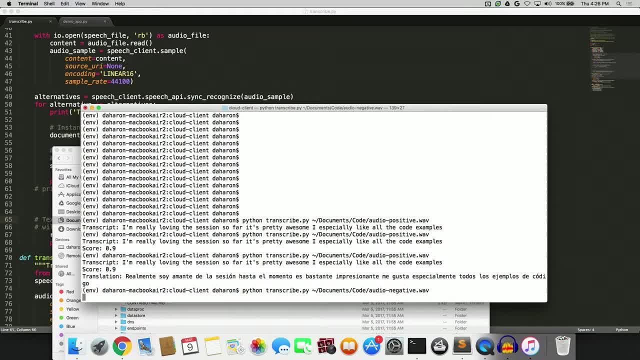 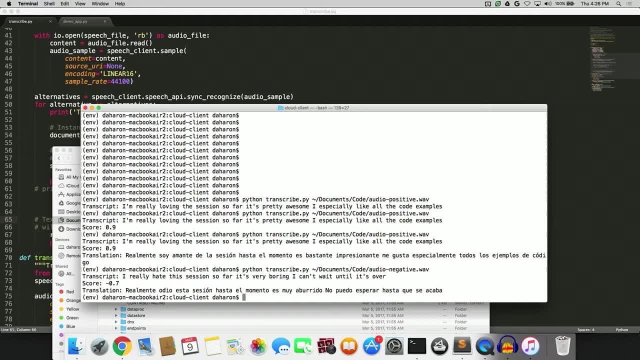 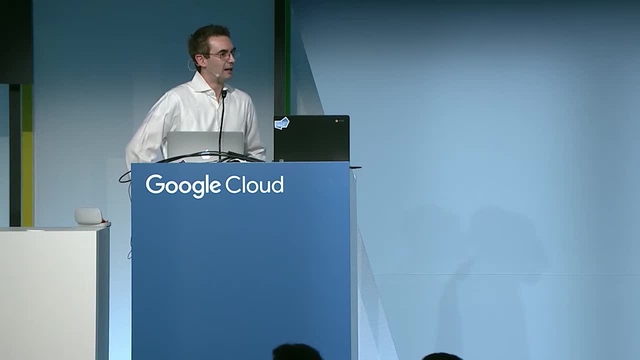 Thank you. So it's pretty awesome And you know This is our beta version. As I mentioned, we're going to have our GA version coming out soon and it's going to be It's going to be even better. 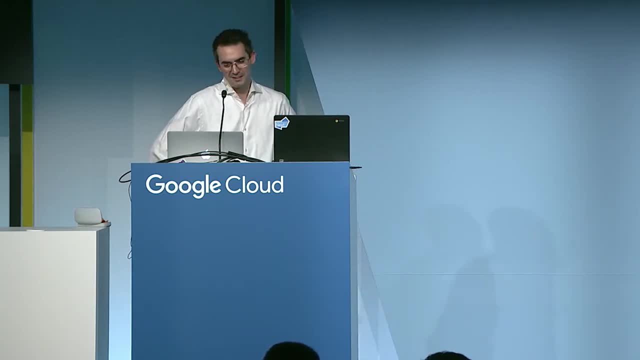 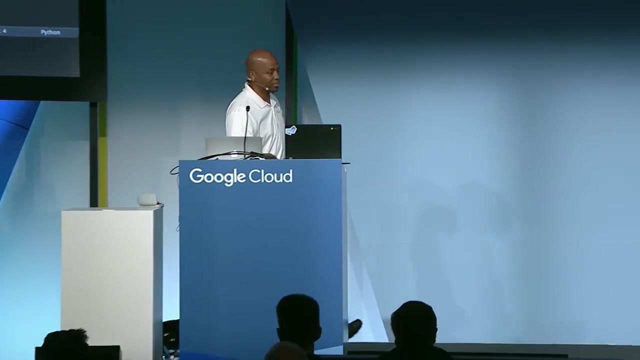 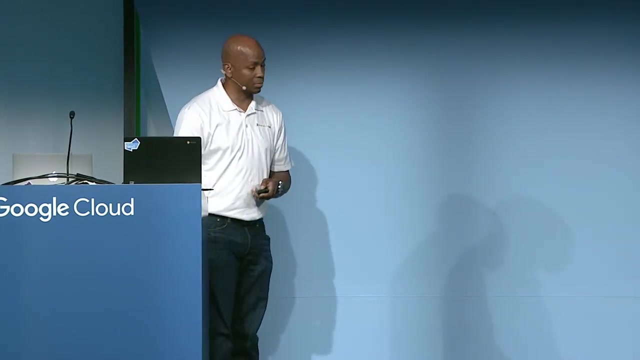 Yeah, I can't go into it too much details, but we're very excited about it. So with that, let me welcome onto the stage Gary from InteractiveTel. Hello, Hello, Jason, If we can go back to the slides please. 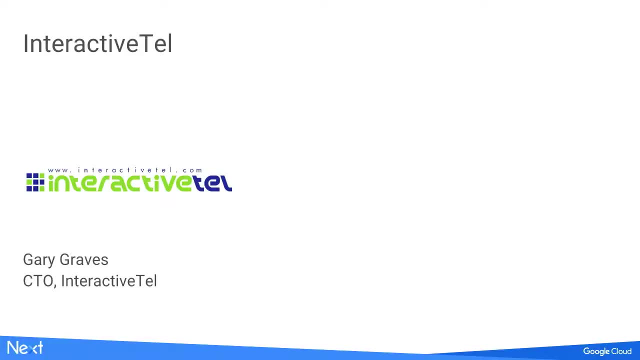 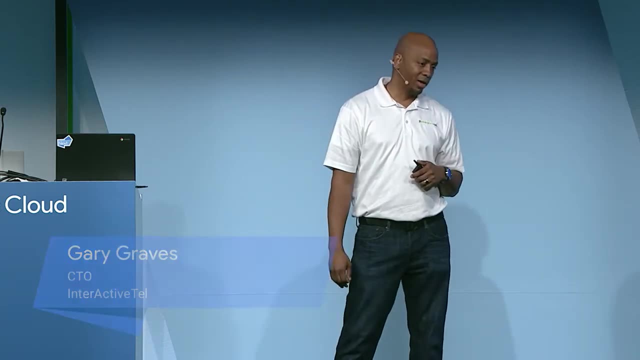 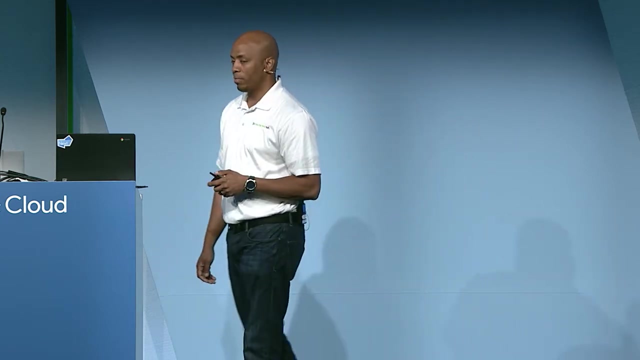 Interact-a-tell provides services to capture and analyze business communications. A lot of the data we collect is audio from the recording of phone calls. We have clients that accumulate a quarter of a million minutes in one month of conversations. To put that in perspective, it would take one person 173 days of continuous listening. 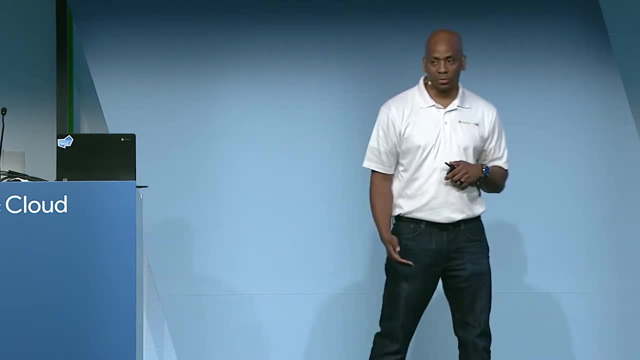 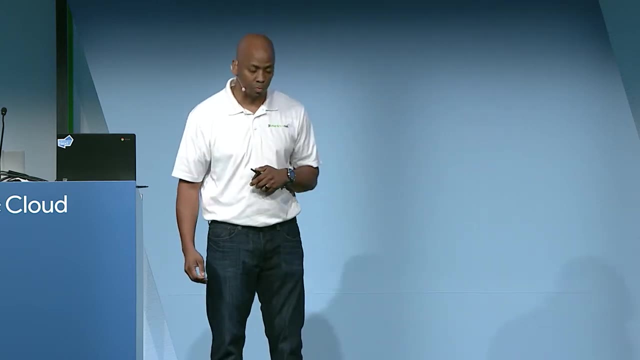 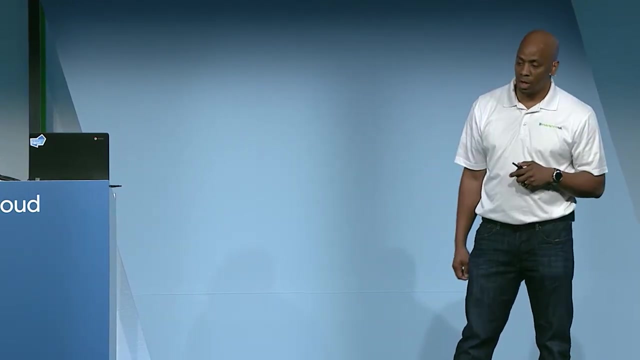 to review every call Now. normally those recordings would just sit there until something happened that caused a particular conversation to come under scrutiny. When that conversation went under scrutiny, it may be because of a disgruntled customer or even a lawsuit. Services like the ones I'll show you today transfer information from a phone call to 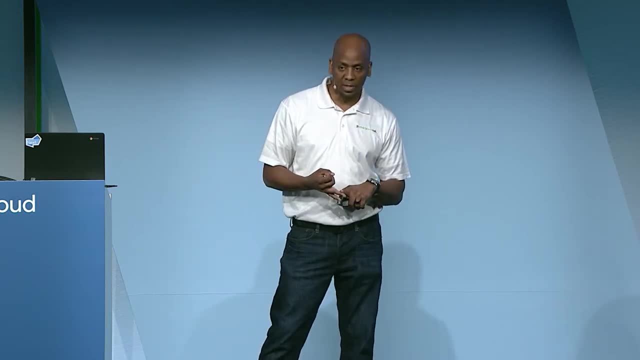 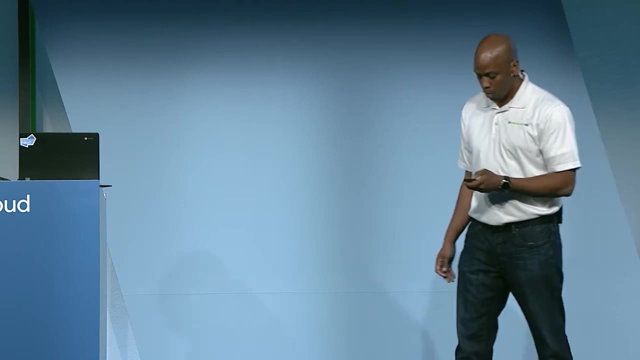 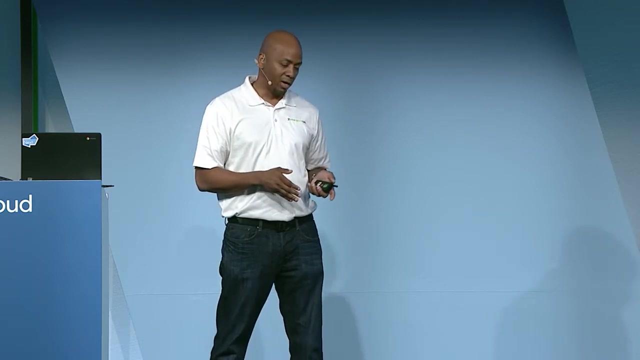 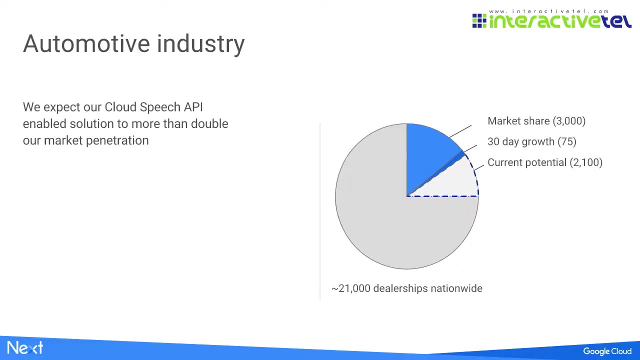 CRM companies to lead and contact management systems, and even to managers, in the form of a text message when something goes wrong. We're able to provide this value by translating speech into text using cloud speech API and provide value to our clients, Okay. 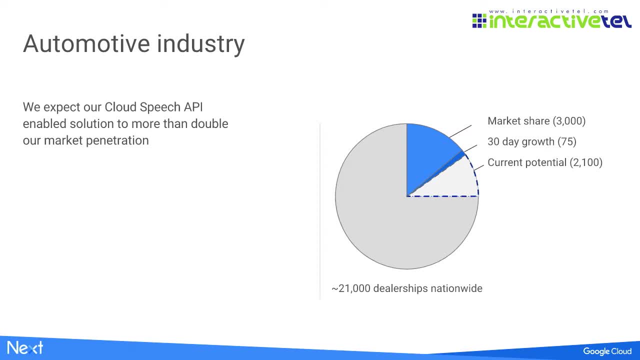 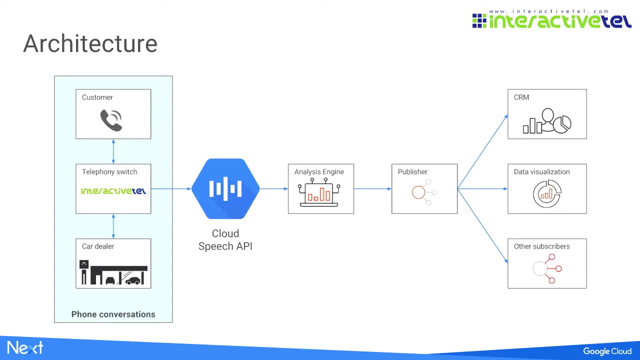 Since the new services we've been able to provide. we've been able to add 75 new accounts in 30 days and over 2,100 new opportunities just from these new services. Let's talk a little bit about the architecture that we use. 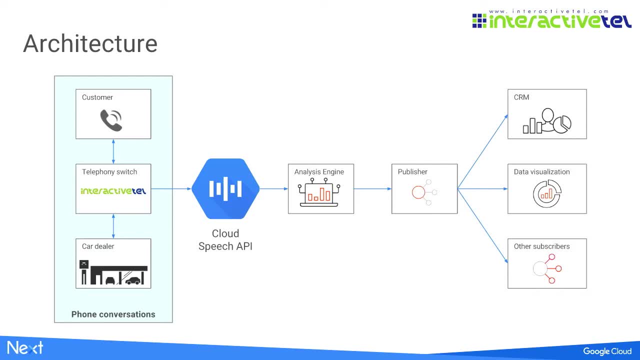 From our telephony infrastructure. we stream speech in real time through Google's Cloud Speech API. We take the results we got from Google and then pass them through our analysis engine, which extracts sentiment, keywords and key phrases, all of which are used to construct. 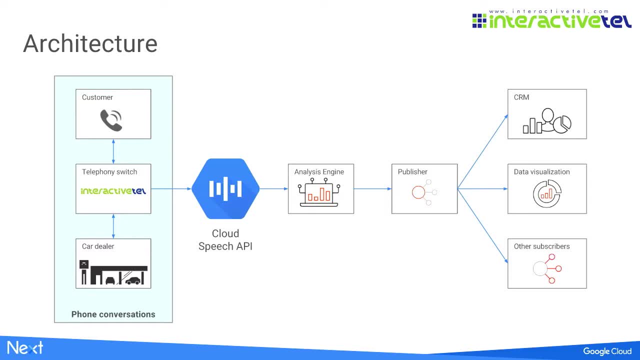 an understanding of what's happening on a call. We take our findings and then publish them to CRM companies, our data visualization tools and other subscribers. They take that information and then pass it along to managers who can intervene if necessary and analyze the data to see what's happening. 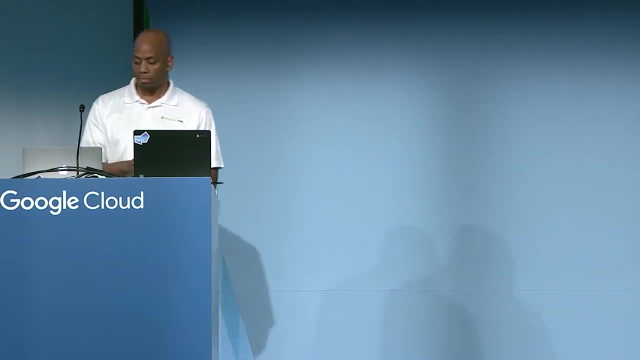 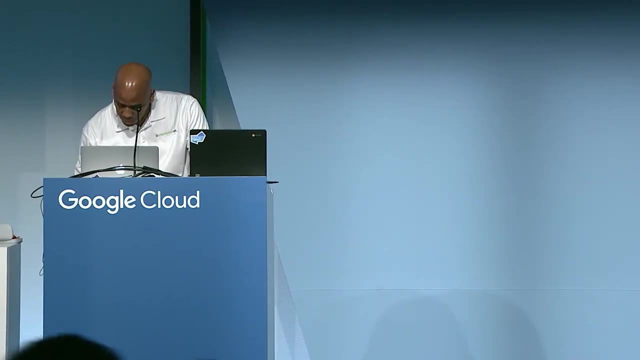 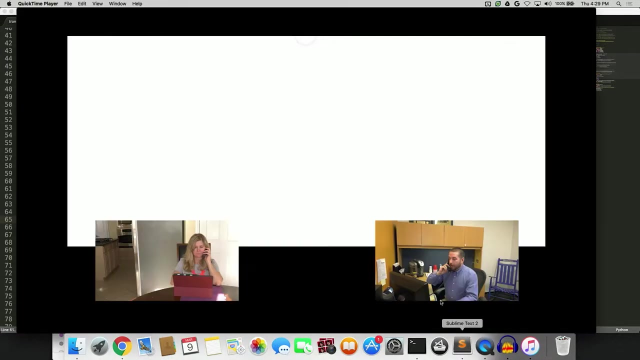 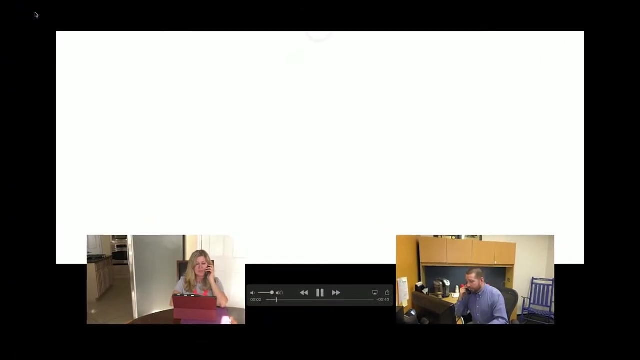 If we could go to the laptop. now I'm going to share with you a video of exactly what happens in a dealership when this technology is in use. Thank you for calling ABC Motors. This is Jack. How may I help you, Hi? 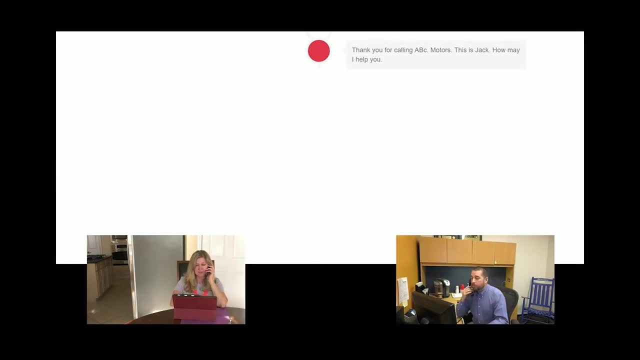 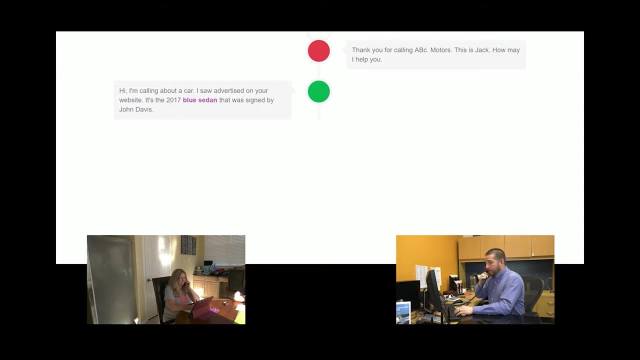 I'm calling about a car I saw advertised on your website. It's the 2017 Lucifer. It's a new car. It's a sedan that was signed by John Davis. Yes, we've received several calls on that car. It's really one of a kind. 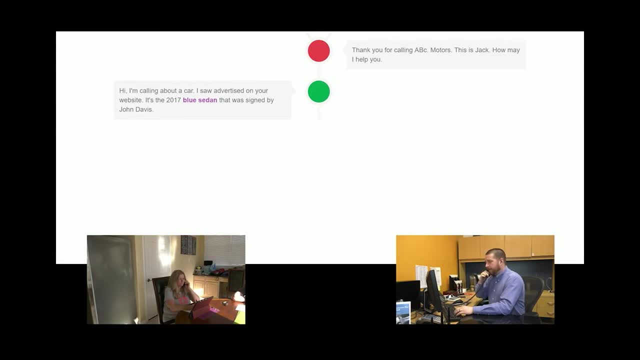 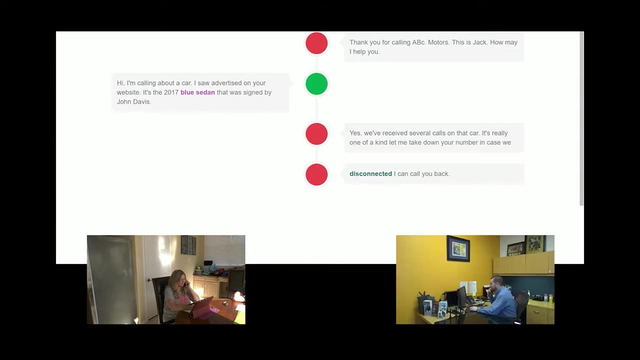 Let me take that out of your number in case we get disconnected and I can call you back. I don't mean to be rude, but I don't want to give out my number. I'm just interested in the car. Can you tell me if it's still available? 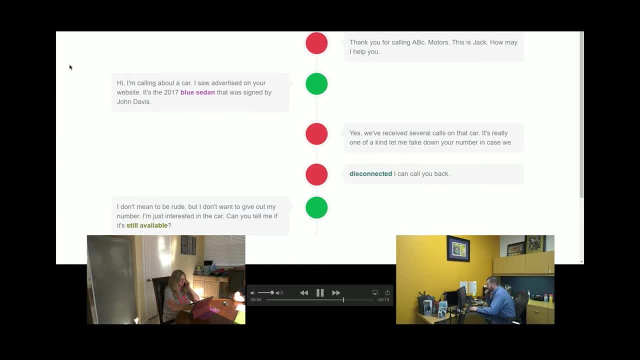 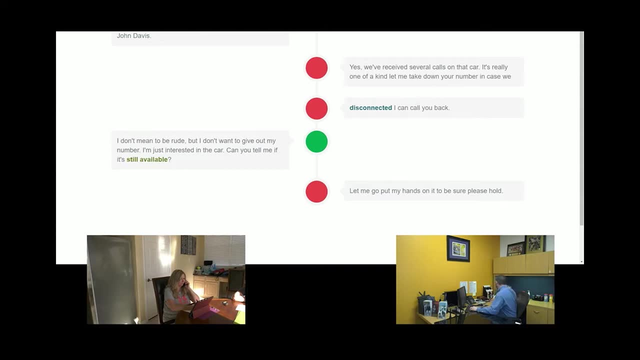 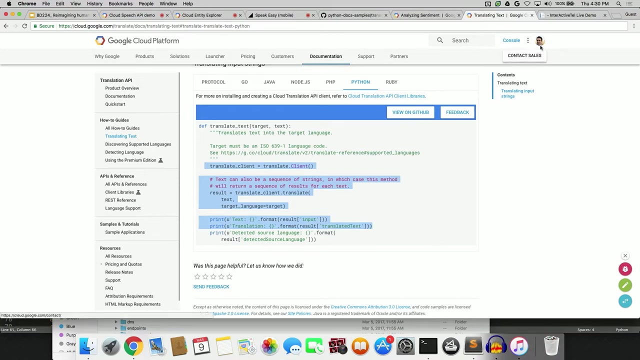 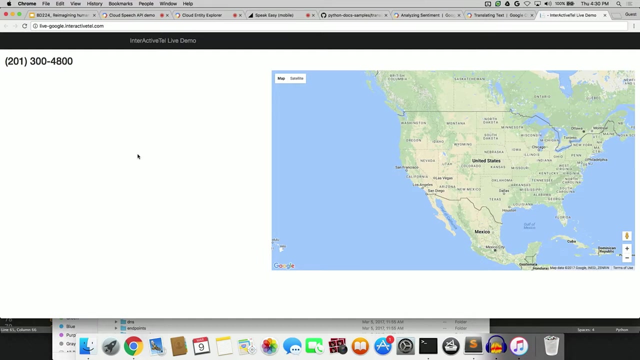 Let me go put my hands on it to be sure, Please hold. I also came up with a nice demonstration for you guys, which is going to require some participation. It sure is On your part. Our specialty is business communications capturing and analysis, so we thought it would. 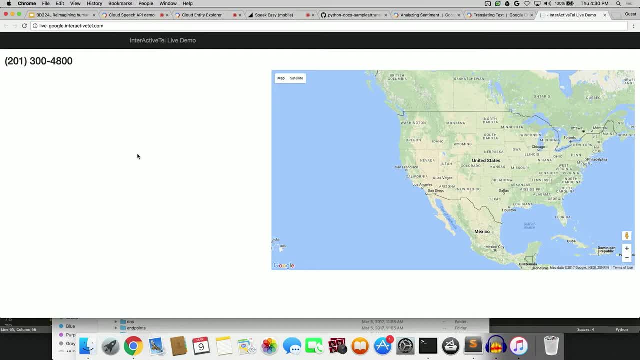 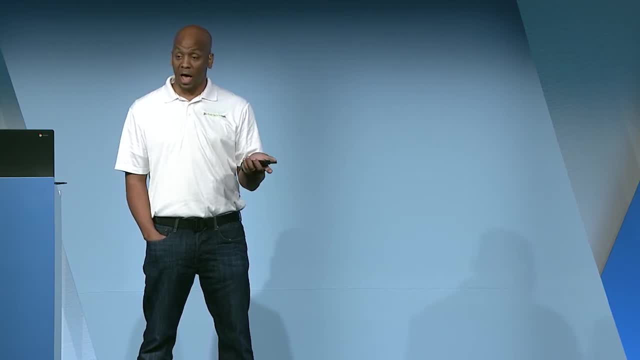 be pretty cool for this demo to have members of the audience call a number which represents the telephony portion We tie into Google Cloud Speech API. We'll ask you where you're from. You mention your country, city, state or what have you. 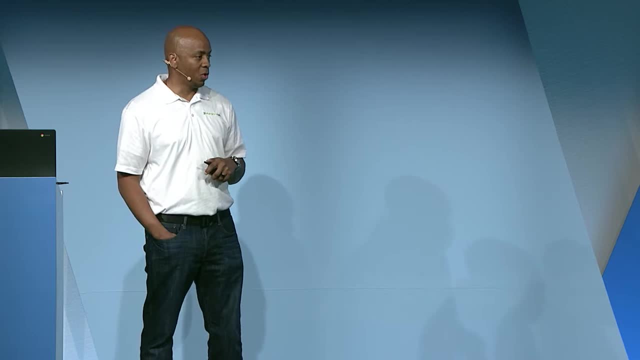 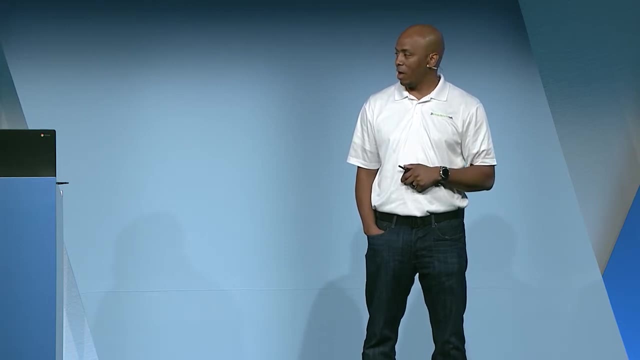 And we'll plot that on the map. So the number that's on the screen: 201-300-4800.. For any willing participant out there, if you pick up your cell phone, make that call, You'll be prompted to say where you're from and hopefully we'll get enough participation. 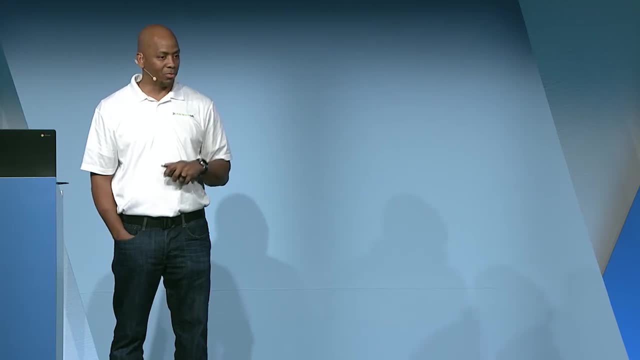 that we'll start getting some blips up there on the map. So, if you will, please make some calls. OK, That's enough of the things we're going to talk about. Who else is here? Who else is here? Awesome? 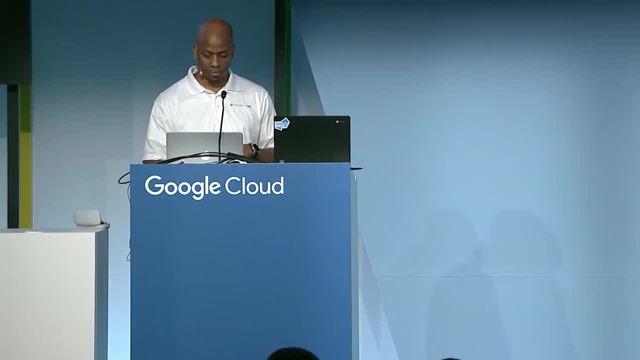 Who else? Who else Visitors, Something else? Who else Must be someone. Who else is here? Yeah, So there are a lot of things here. There's a lot of questions. It's just a little while You have to go through the questions. 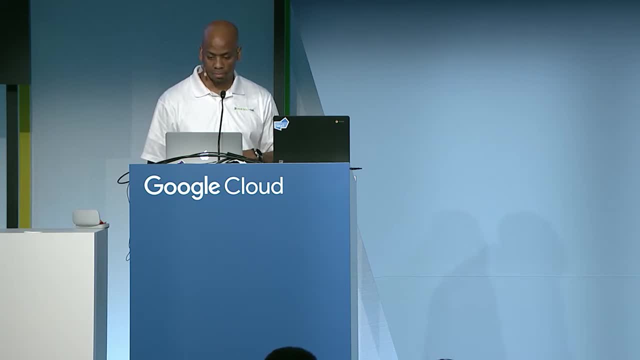 Yeah, Sorry, I don't know. I don't have time, so I'm going to get into the question. So, basically, how do you work with these people? I'm just going to basically pick a question. It's a list. 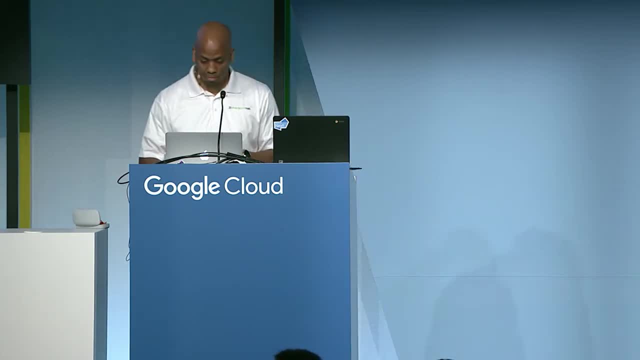 There's a lot of questions. How do you go through these questions? I will give you a list of things. So that's interesting Questions. So this is using gRPC to stream in real time while you guys are on the phone and you'll. 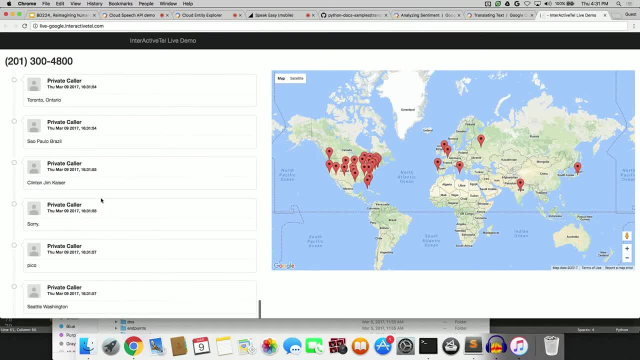 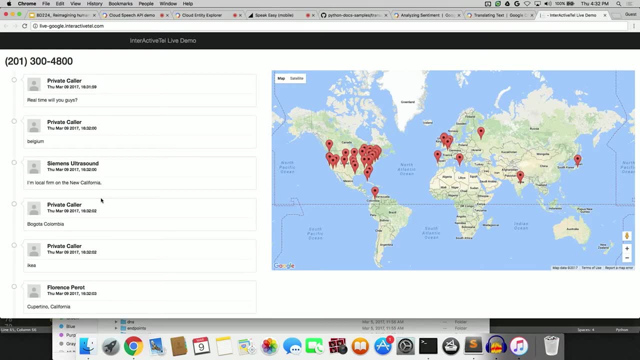 notice a lot of names are popping up there. We're doing reverse phone append to also attach additional value. What's also interesting about this particular mashup is if you don't say a city or state and you say a particular company, if that company is, you know, has a presence on Google. 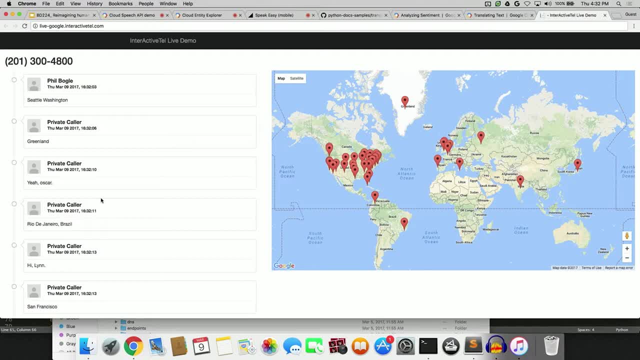 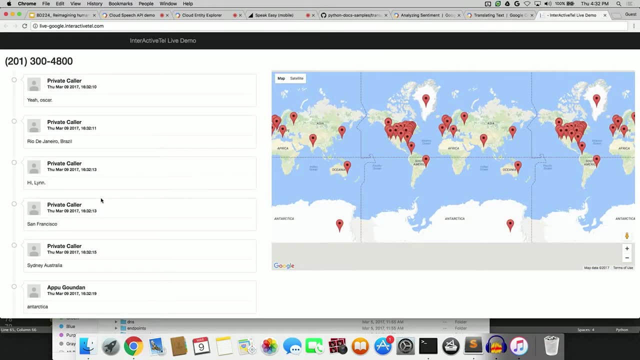 Maps that would also show a dot there. We'll leave this up for probably for the rest of the day. so if anybody was savvy enough to copy the URL, the phone number, this demo will be active for the remainder of the day. 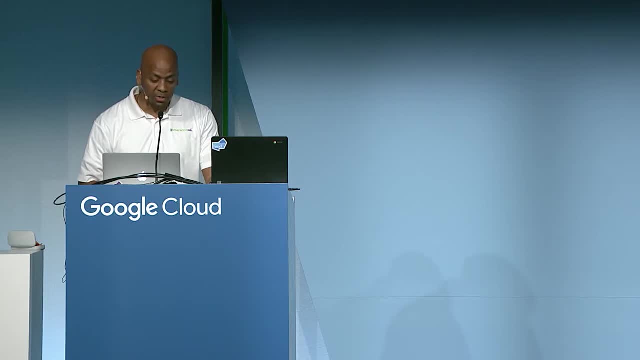 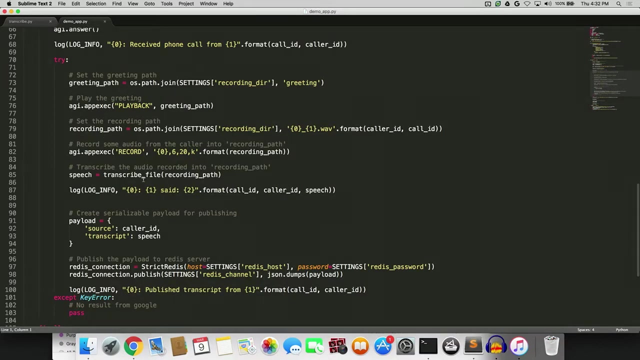 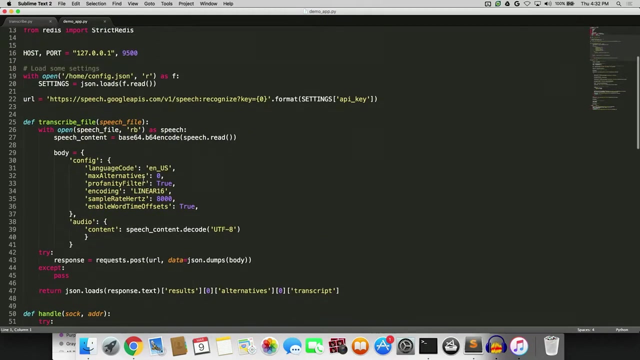 I'm going to transition into the code behind this particular demo. It's very similar to what Dan showed earlier Effectively. you know this is telephony code where we're playing greetings recording the file locally And the transcribe function is very transcribe file function is very similar to the one that 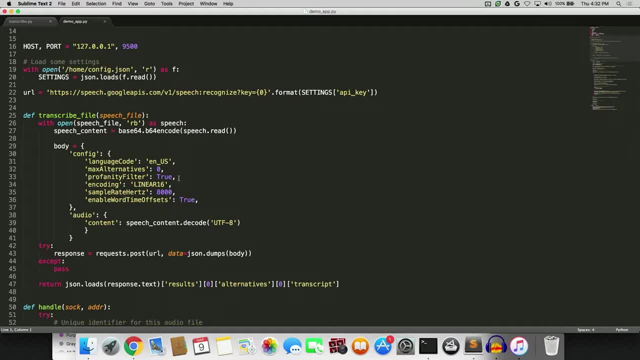 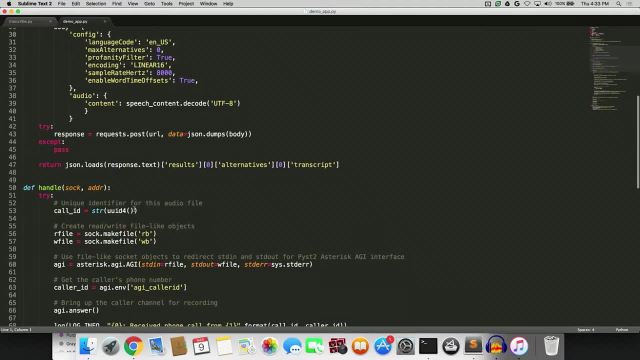 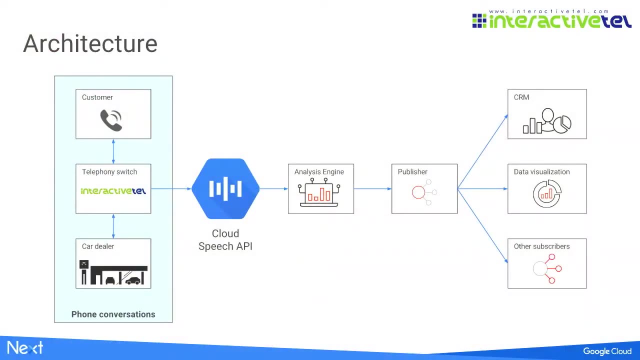 Dan showed earlier. Of course, we've enabled the profanity filter to make the results less interesting. If we can go back to the slides, please, We do have a couple of things that we want to talk about. First of all, we want to make sure that we're using the right code. 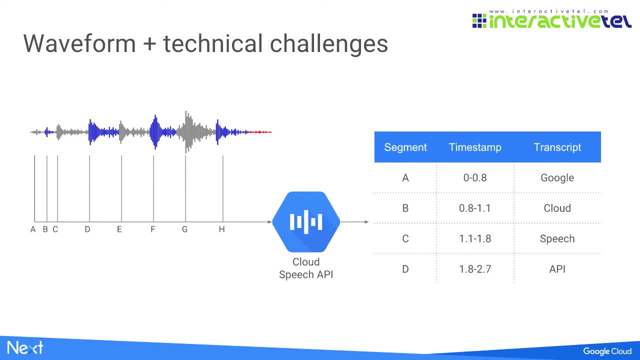 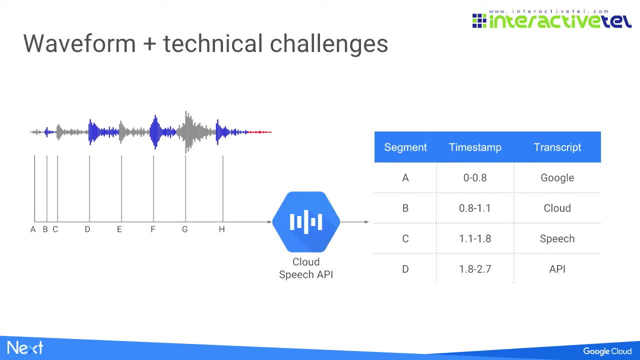 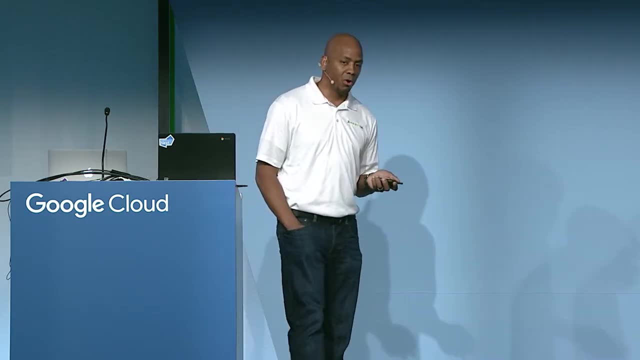 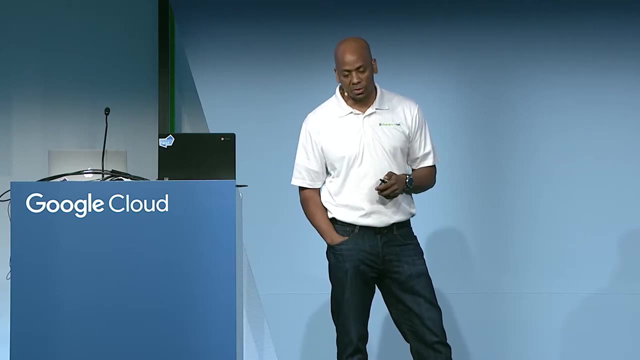 The first of which was timestamps, And I don't know if any of you are here- are part of the user groups, but that's a topic that came up quite frequently. Many phone calls are 15 minutes or longer in length, And an important part of our user experience is allowing a person to click on a keyword. 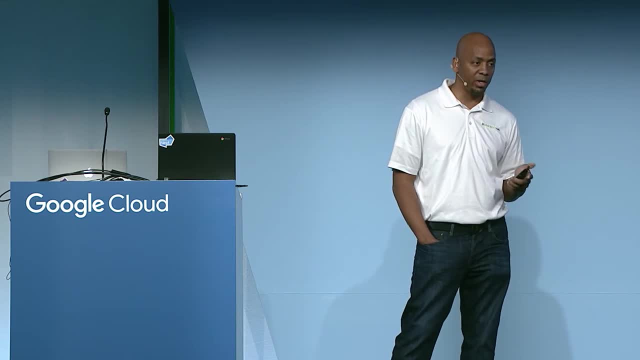 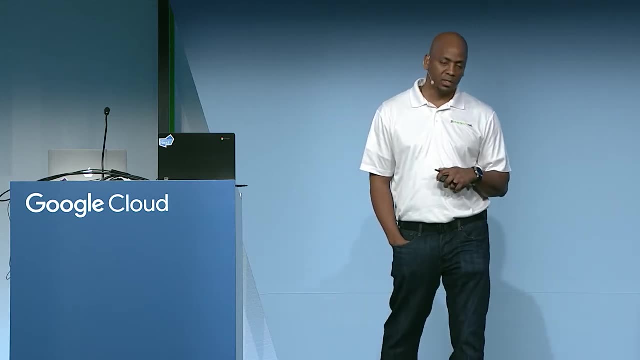 or phrase and skip ahead to a phone conversation to the point at which that word or phrase was spoken. Currently, Cloud Speech API does not provide timestamps, but we did devise a way to implement them that works for us. The way we did this is as follows. 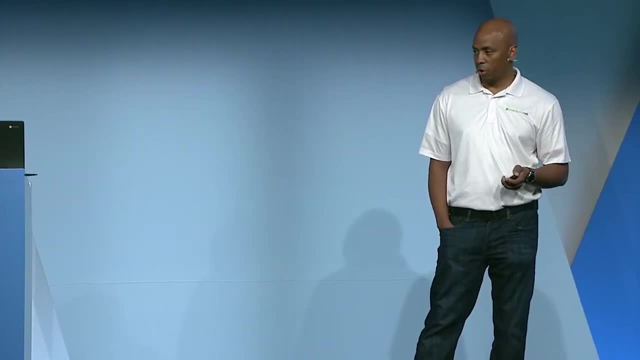 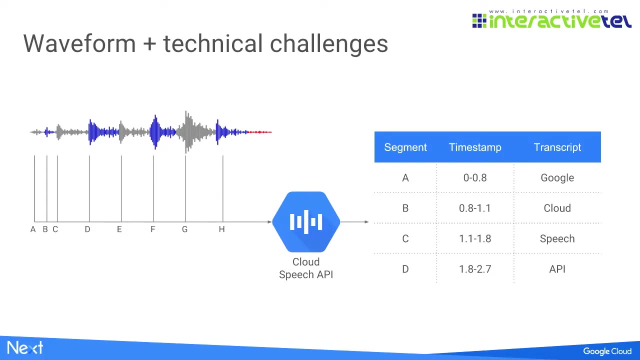 We pre-processed the audio to detect silence in between words and phrases. We then used that detected silence to segment the file and submit those segments individually to Cloud API. The responses we get back we associate with the segment and the interval at which we detected. 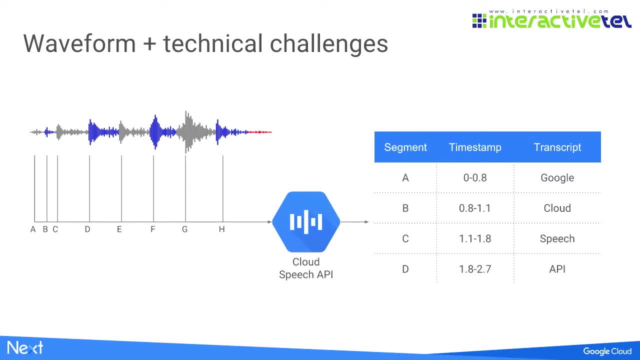 and it allows us to know that, for instance, segment A, which comprised the first eight tenths of the conversation, was the word Google. We repeat that process for each word or phrase in the recording and it enables us to construct a transcription of exactly what happened on the call and the time in which it occurred. 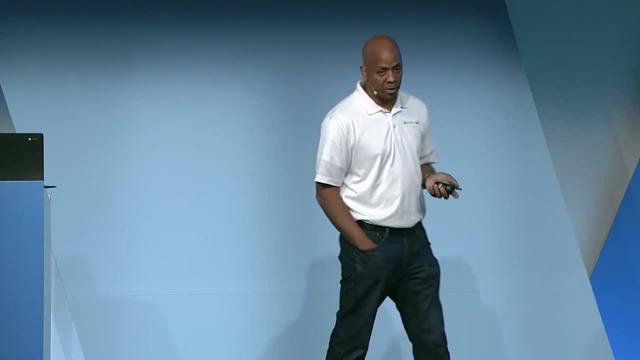 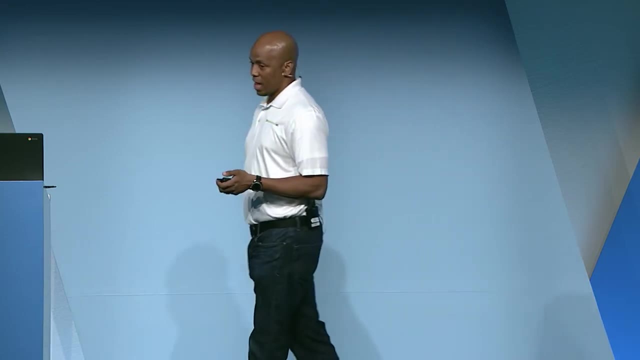 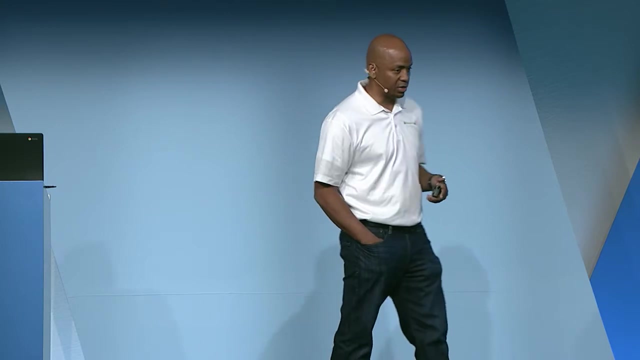 Another issue we ran into was speaker diarization. As we're a telephony company, we have two sides of the conversation. Cloud Speech wasn't really designed initially for this type of conversation, so we record our files in stereo, which gives us a caller on one channel and the callee on the other. 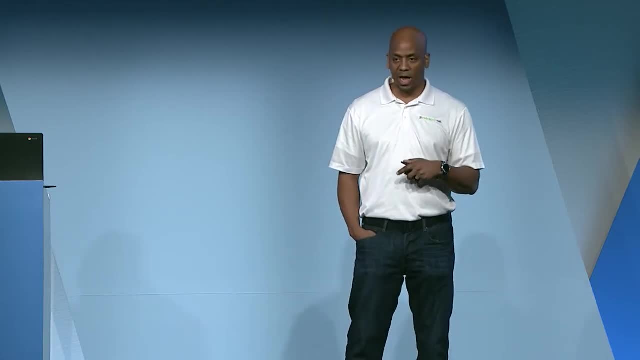 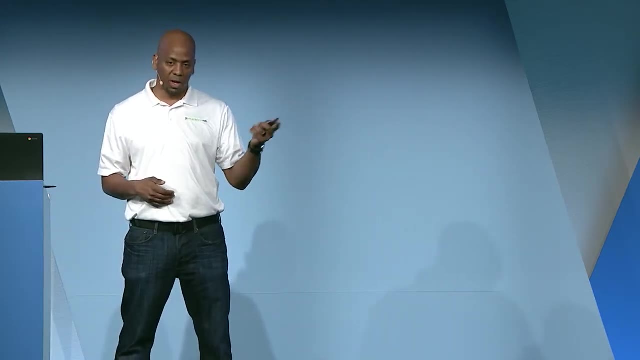 Now, if we were to take that audio file and separate them into two channels, we'd end up with one minute of audio, one minute of phone call and two minutes of audio- one minute for the left side, one minute for the right- effectively doubling our cost for processing. 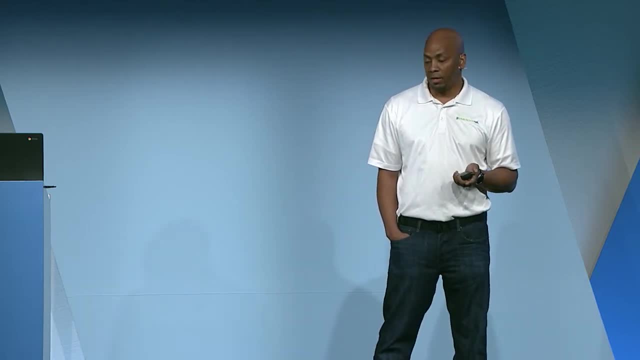 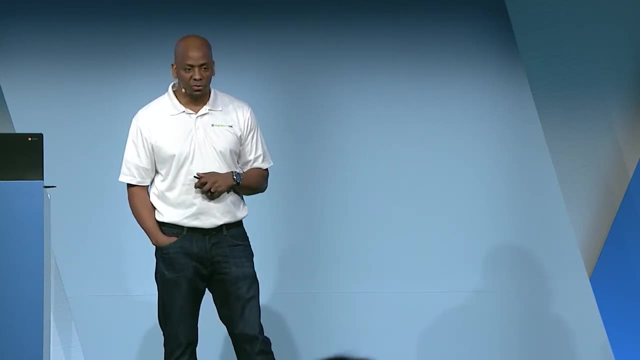 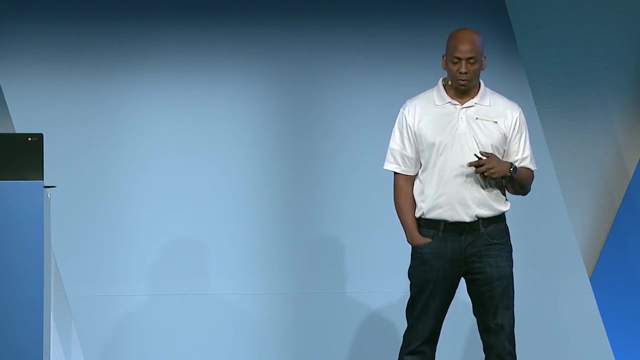 a stereo file. In order to mitigate that, we expanded our pre-processing algorithm to detect large spans of silence. We then remove that silence from the audio and submit the segments individually, keeping track of whether that was submitted for the left side or the right side of the conversation. 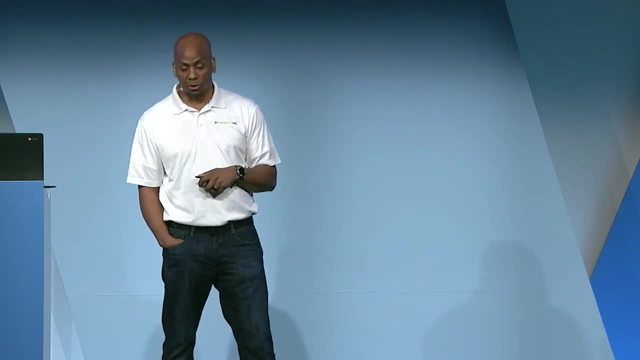 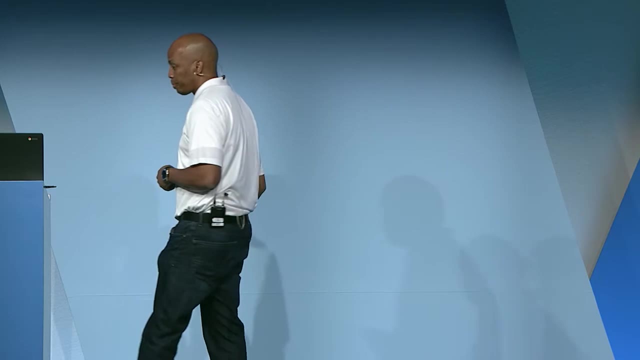 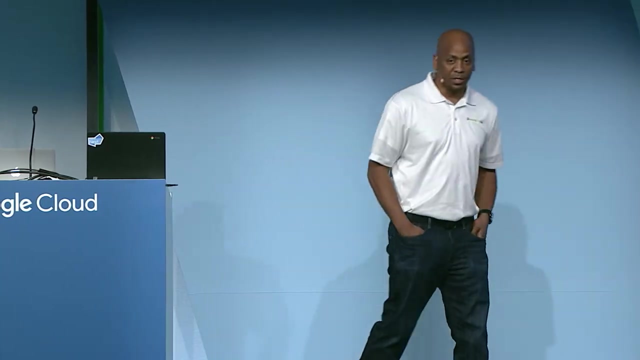 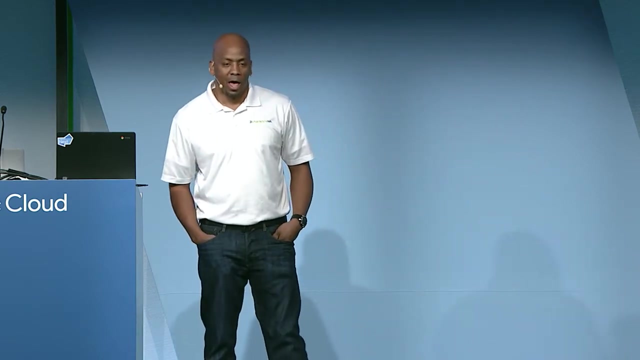 We then reconstruct the transcription using the method that I showed you earlier. In this case, we're associating segments with time intervals, but also associating them with the caller or callee. Our experience with Cloud Speech API has been pretty awesome. I learned a term yesterday, which is dark data. 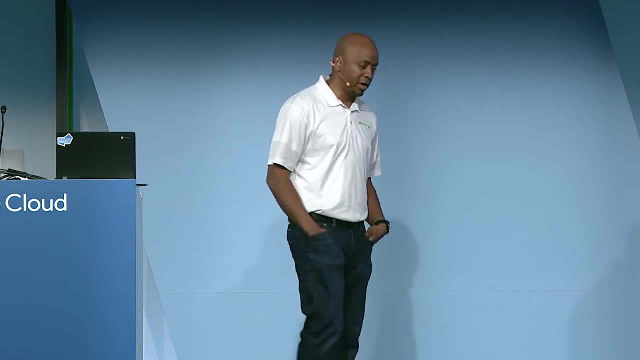 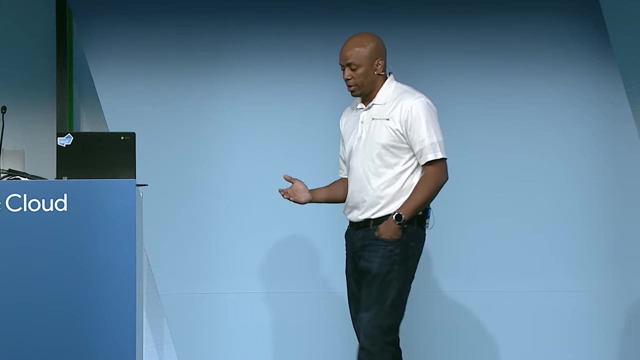 For us recordings and for probably a lot of you that may have audio. that happens today in recording format. it's just dark data. You don't know what's happening. You don't know what's going on there. Well, using Cloud Speech API, we were able to shed light on our recordings, and I'd like 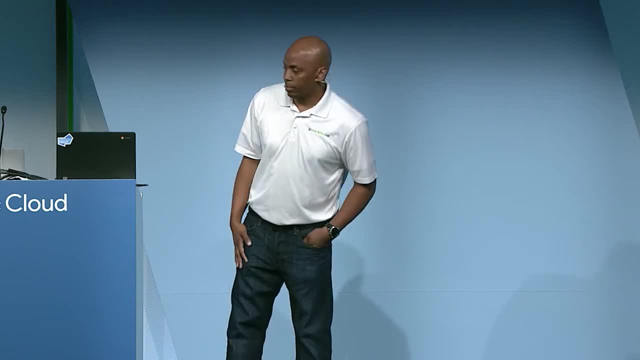 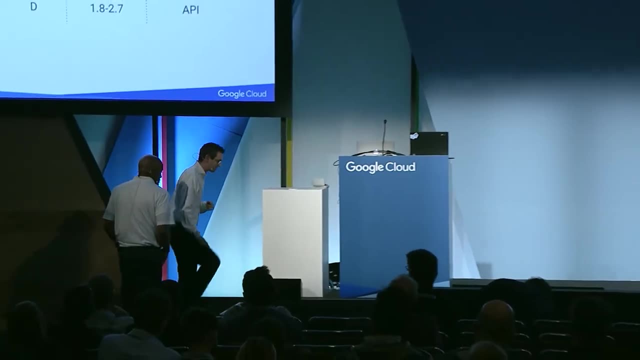 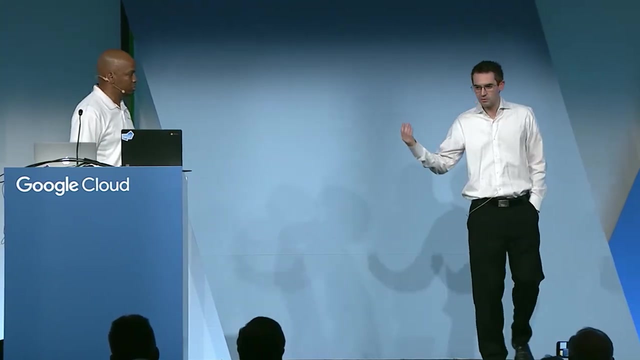 to thank you for allowing me to share that experience with you. Maybe, if you can stay on stage, Gary, I actually have a question for you. Could you talk a little bit about once you transcribe these phone calls, for example, that scenario that you showed in the video. 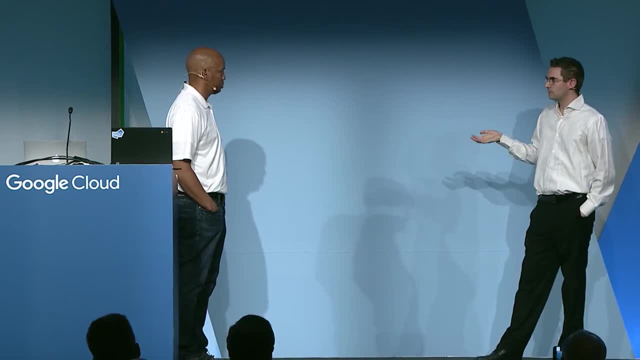 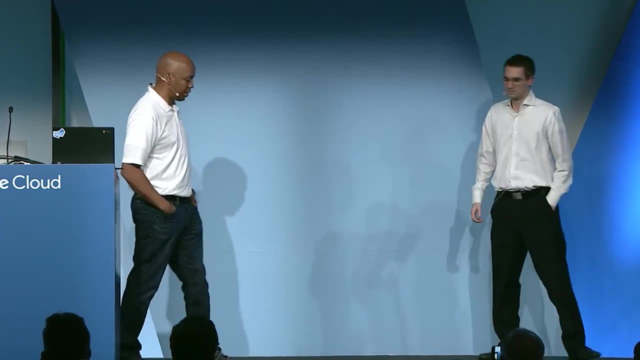 Where a customer is calling about a car that's not in stock. What do you guys do in terms of the analytics, in terms of the workflow? How do you provide value to car dealerships? That's a great question. Example is: you see a car on a website. 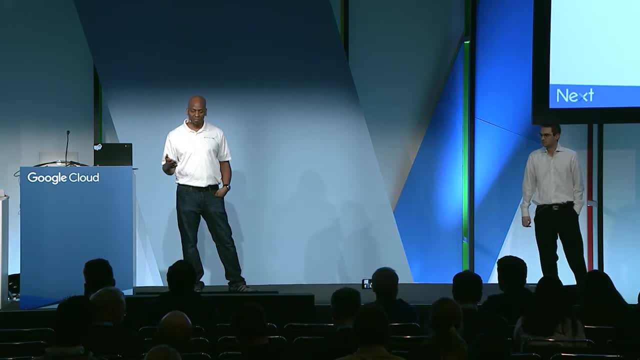 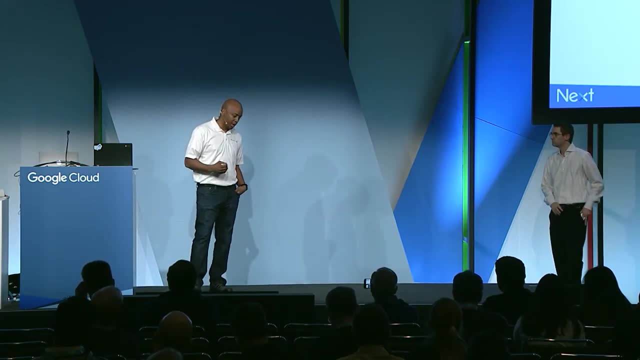 You call in and, for whatever reason, that car is not available. This particular dealership is using our system, so we know exactly what's happening on the call. In the automotive space they have a notion of everybody that calls in you want to get. 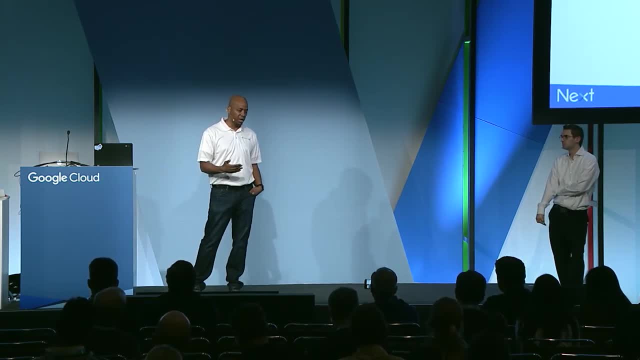 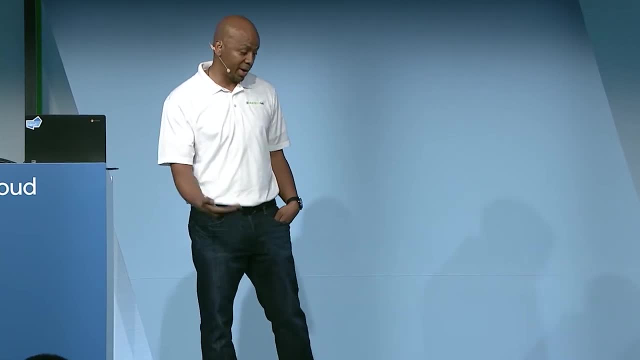 their contact information, their name, their number, product of interest- so that if that product does become available- because it's a very fluid market- you have a point of contact to reach back out to them. So we identified a couple key factors. 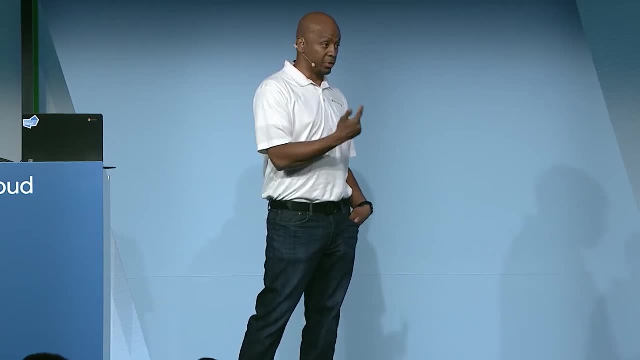 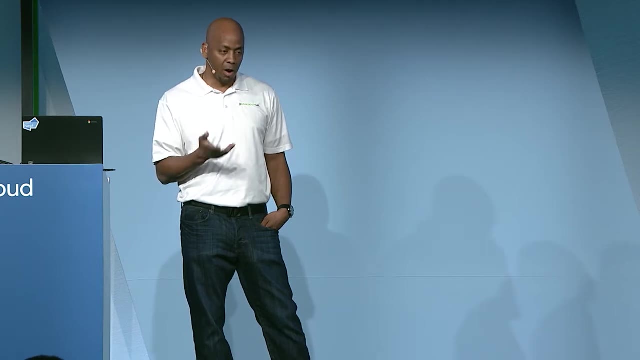 Number one: the call was for sales. Number two, there was a product that they were interested in. And number three, there was no contact information that was collected In our space. we call that a missed opportunity, which becomes actionable because we'll send. 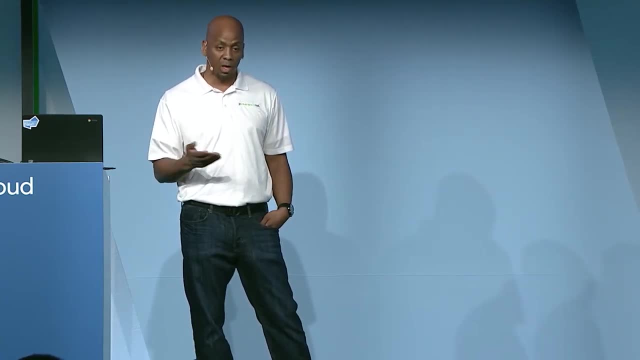 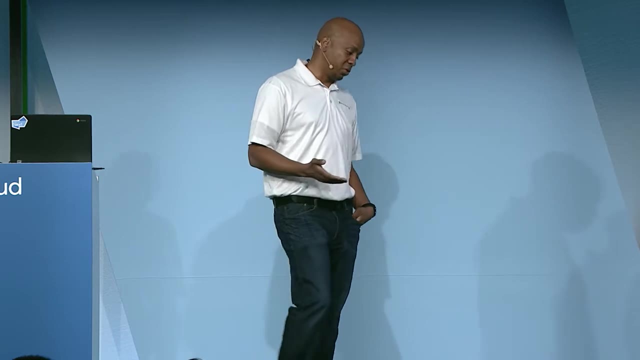 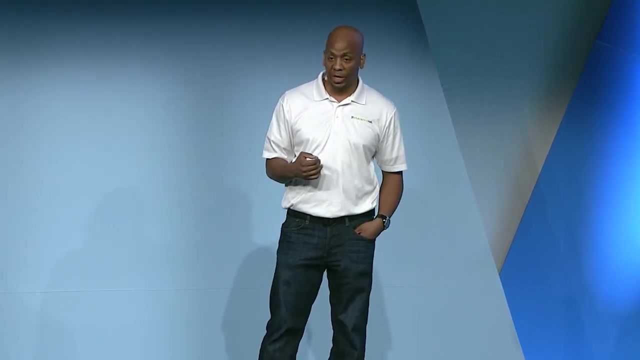 that to a sales manager, in the form of a text message and or an email based on his settings, to let him know that this particular opportunity may have been missed. What ends up happening in those cases? large dealerships have this instance occurring dozens of times a week and it really impacts their bottom line to be able to have a second chance. 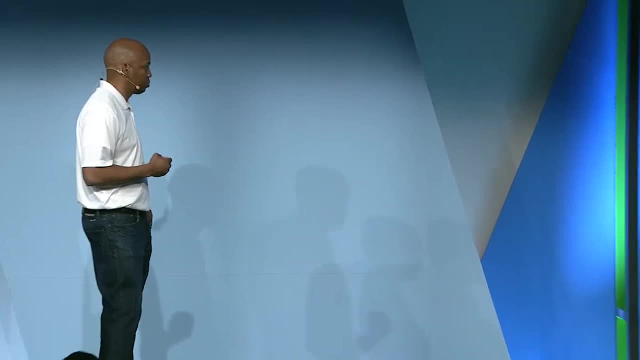 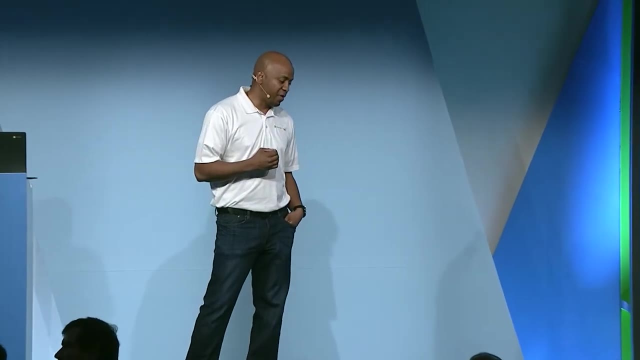 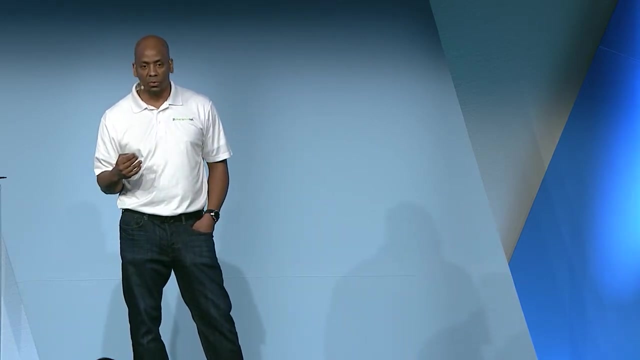 at selling that particular customer. So what have been reactions for dealerships that have tried the new system? Well, the reaction has been overwhelming. In fact, large dealer groups that we've demoed and had an opportunity to show our system to end up pushing it out throughout their whole group. 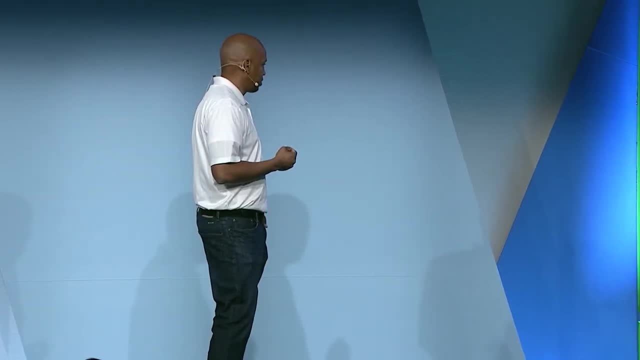 I don't know if I'm allowed to mention customer names, or I mean if you can just say like, in terms of business value, like are they actually making more sales, or is this just like a nice-to-have? 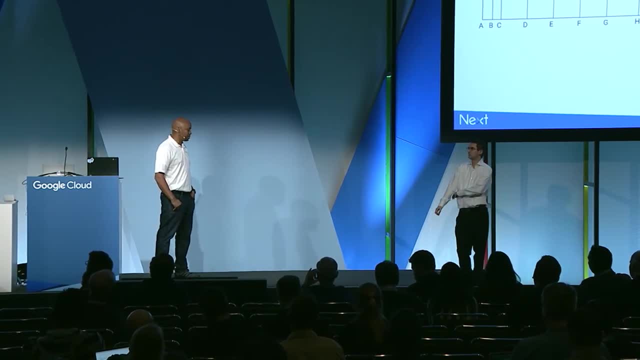 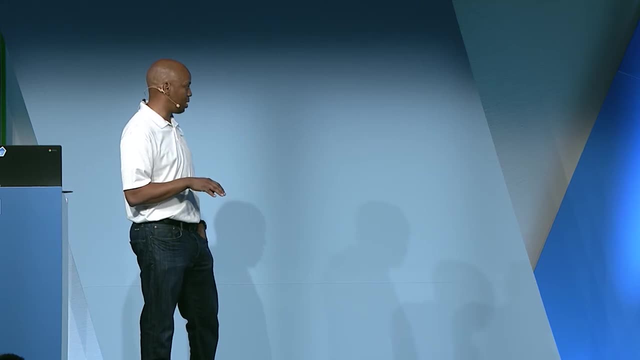 Well, not only are they making more sales, but it's causing a shift in the mentality at car dealerships, And that's because now everyone in the dealership is being held accountable. It's one thing to have a recording or monitoring solution in place, and people know it's there. 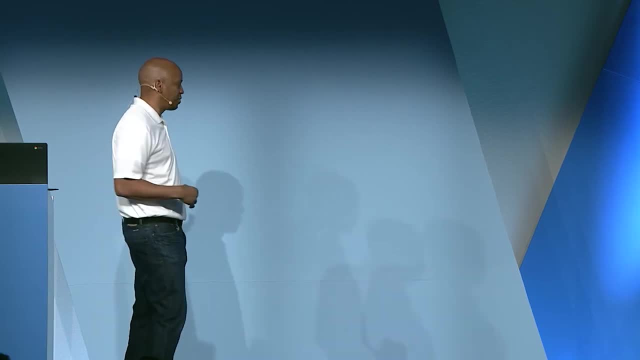 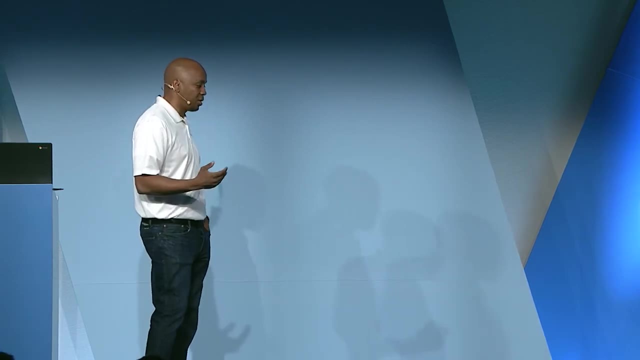 but that's reactive, meaning the only time that that information is ever going to be leveraged is if there's a situation that calls that into question, Whereas, using cloud speech, we're able to mine these conversations for actionable intelligence to allow us to empower dealers to be proactive and provide a higher-level service to our 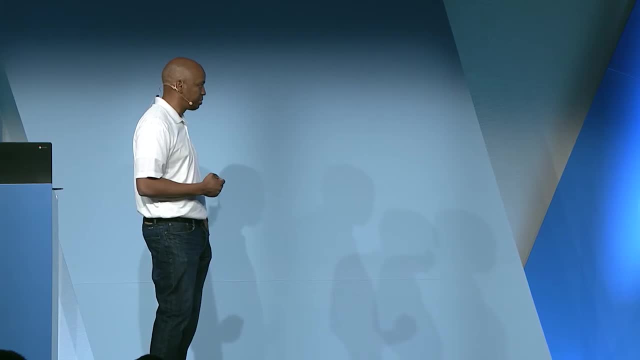 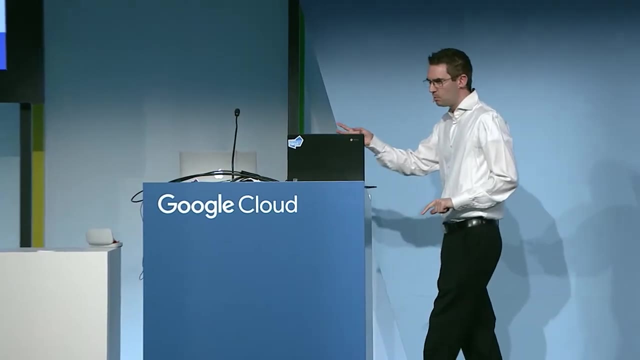 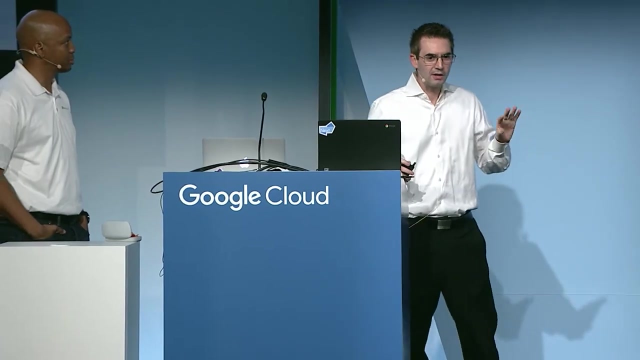 customers and it's really becoming disruptive in our industry. Great, Awesome, You can stay here. I just have two more slides and then we can do Q&A, So I just want to give you guys a plug for two more sessions that are happening you. 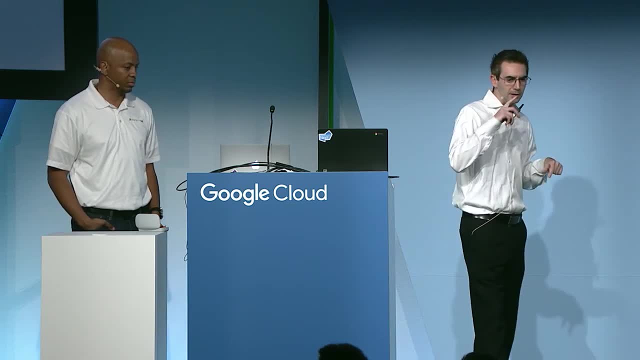 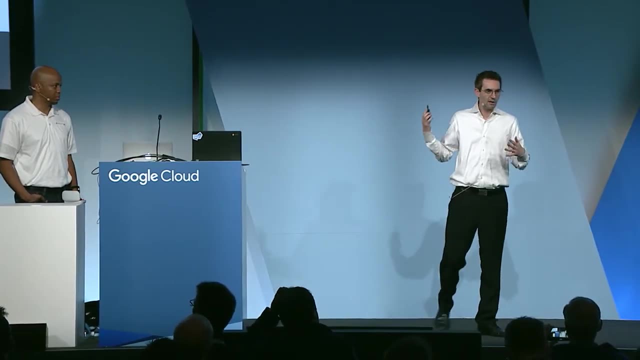 know a little bit after this one in about 30, 40 minutes. One is sensitive data management, So you get all this text coming back from SpeechAPI. A lot of it is going to contain PII. A lot of customers have asked us: what can we do about that?